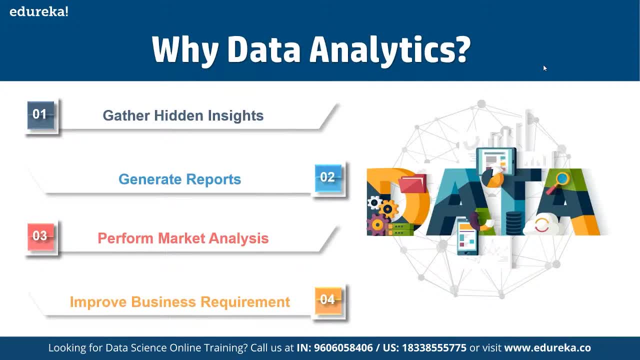 How one data pointer affects the others, and then if they are not able to get the inside, or what exactly is happening with the own user base, how the market is going on and how they stand and they are positioned in the market, They won't be able to sustain. 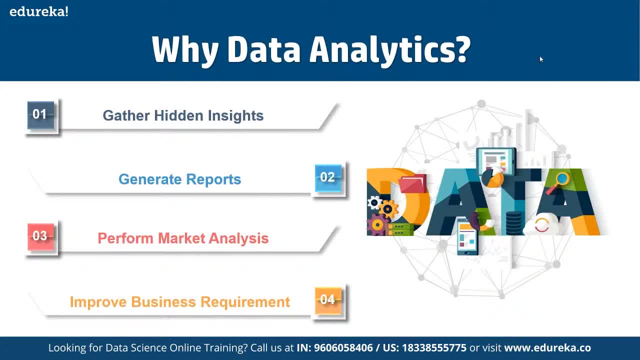 They're positioned in the market for long right, And that exactly is what EDA helps the companies in achieving that. so EDA ensures- and again, not before, even EDA- We, the concept for data answers ensures that they are going to have this answers. 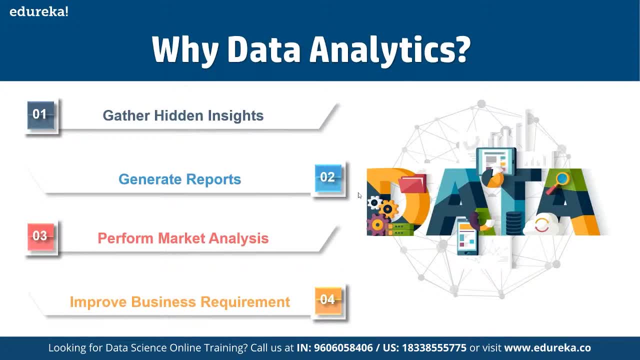 Available to them so they so that they can take a proper actions. So it offers them insight on they've offered them inside. It helps them in generating the report. It helps them in Performing the market analysis and getting a better insight on what exactly is happening. 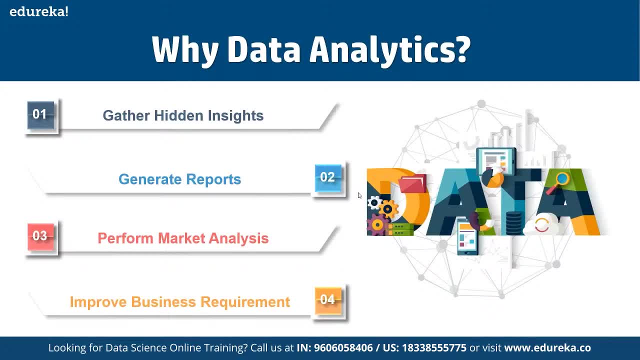 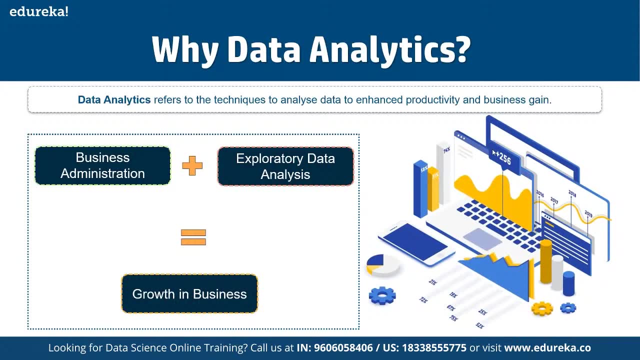 by their own data sets. So if you talk about why data analytics, so data Alice prefers to techniques to analyze data to enhance productivity and business goals. So it involves two different components: business administration and exploratory data analysis, and these two together results in the growth. 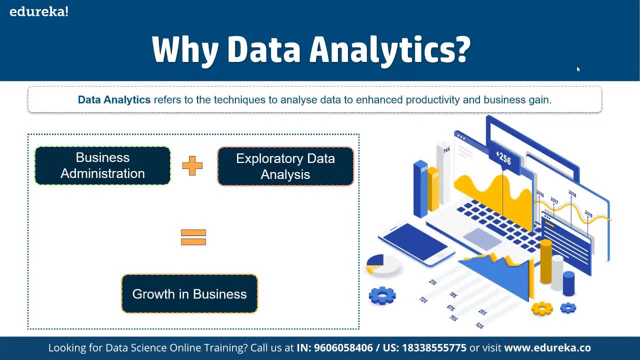 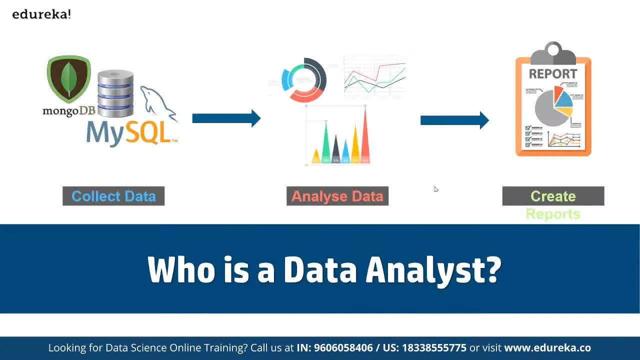 for any business that we can think of. So if you talk about who exactly is a data analyst, so data analyst is someone who is having a good knowledge on performing the ETL activities. When we say ETL, we simply mean extract, transform and load. 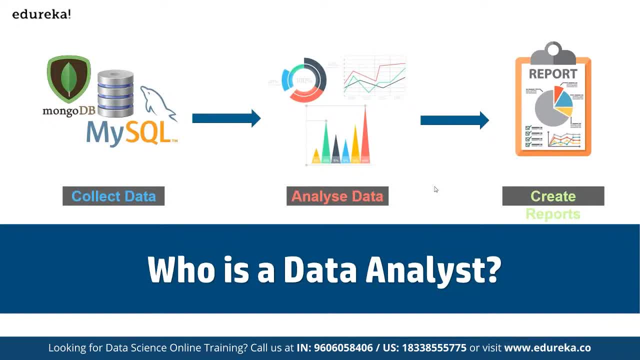 That means we know that data will be scattered in different sources for any company, correct, And we have to make sure we are able to extract data from multiple sources And, for example, we may have data stored in MongoDB in a complete database, or in ERP solutions, in CRM, and we have to, we have to extract data. 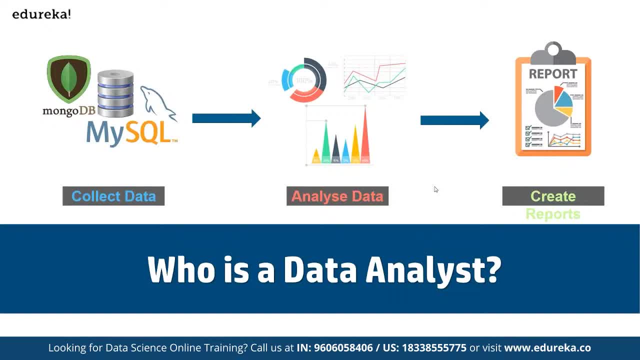 from these different sources, first of all, correct. So we have to work on data collection and then data analyst. They will have to work on data analysis in making sure they are used. They are going to use the right type of visualization to make sure they are able to create a good report. 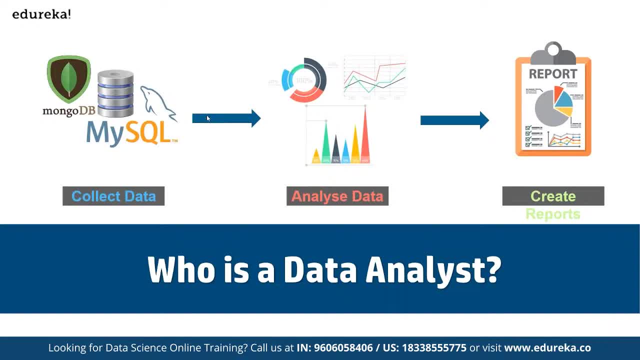 for helping the stakeholders and the other team members and finding a pattern in the given data set, and then they can simply use it for getting a better insight on which the forecast can be generated. same way: here We have to create reports as well. So, based on the entire analysis, the reports they need. 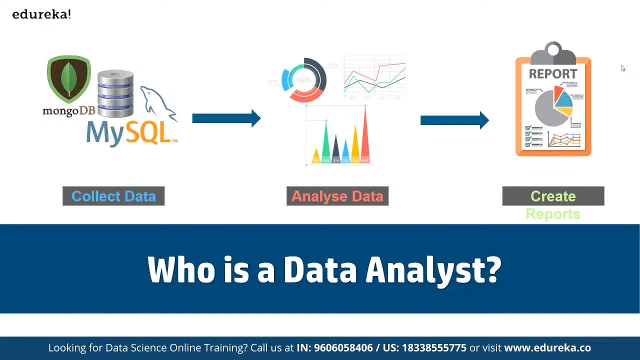 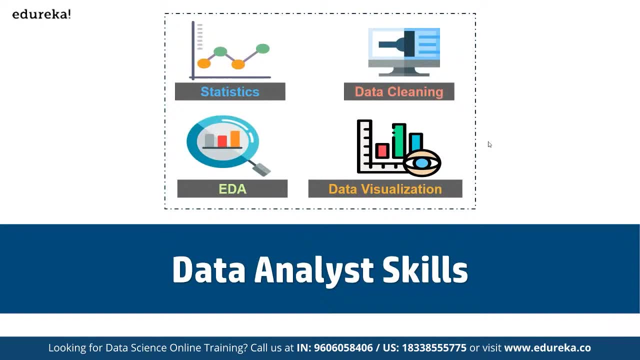 to be generated as a part of the job role for any data analyst And they are responsible to apply these skill sets. So again, any data analyst. they should be good with status, sex, with data cleaning, with the concepts of EDA as an exploratory data analysis. 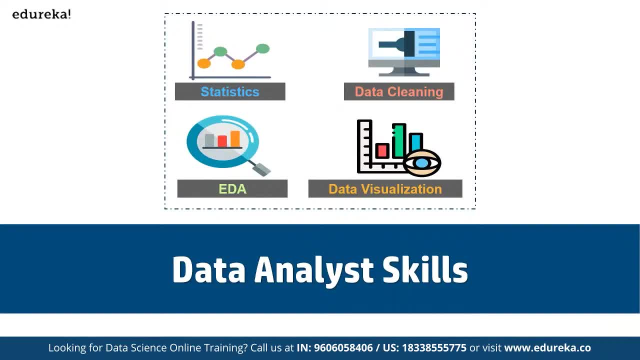 And they should be good with data visualization methods. I mean again, they can also be good with multiple bi tools that we have business intelligence tools, like we have power bi. we have table servers, So they should be good in that one as well, so that they can use these platforms. 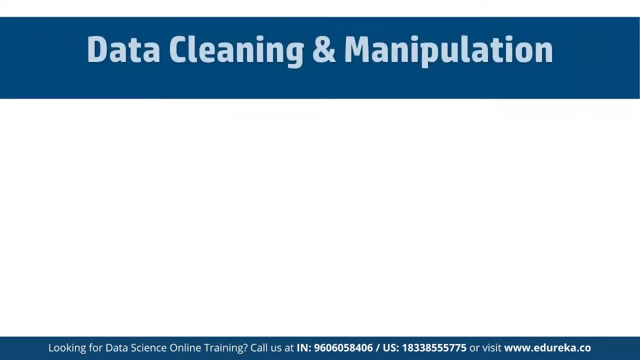 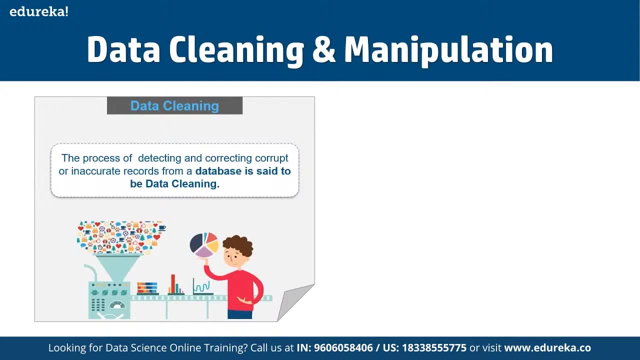 to create the visualization that we need. Now, if you talk about data cleaning and manipulation, Now data cleansing is a part of any data analyst, because the process of detecting and correcting corrupt or inaccurate records from our database is said to be data clearing. now We know that data will be Rob and we are trying to extract data. 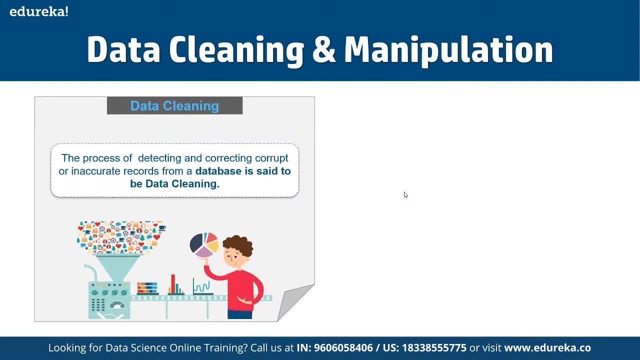 from multiple data sources, right, And any data set will be having multiple anomalies. now, to understand the process of data cleansing in a better way, We can take a small example by referring to our Excel sheet. So let's open up a blank spreadsheet here. 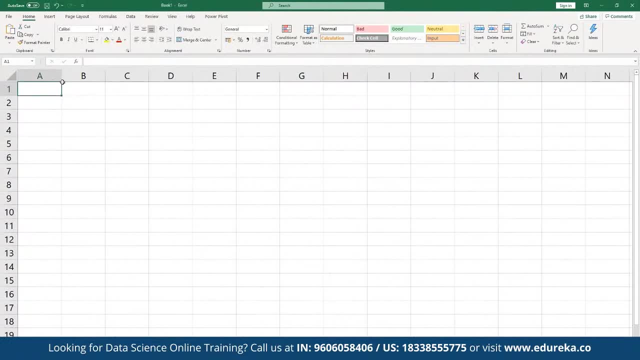 And let's say we have one data with us. For example, let's say, here we have data for product, here We have the product, and then here we have the something called as quantity ordered. Then we have amount paid or can say total amount paid. 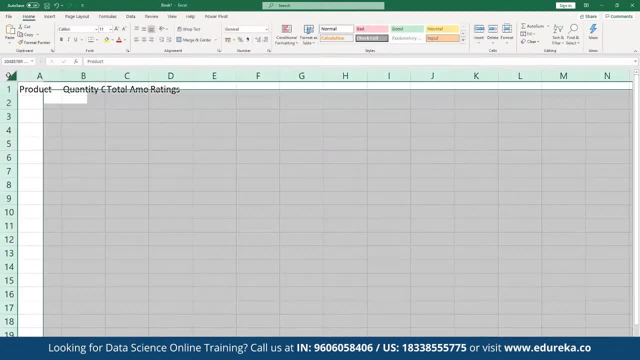 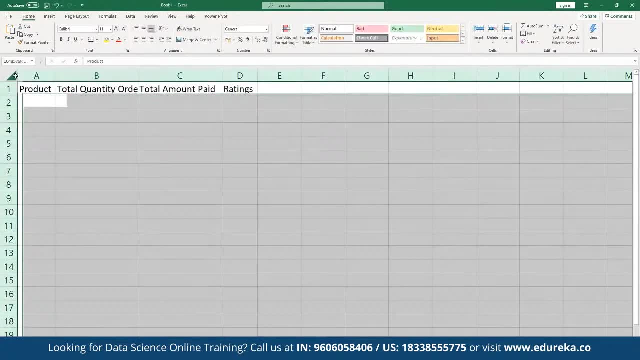 We may have ratings. So let's say, here We have these data pointers available with us, We have total quantity ordered, We had total amount paid, and then we have products and then we have the ratings for it. All right, So let's say, here we have this kind of data with us. 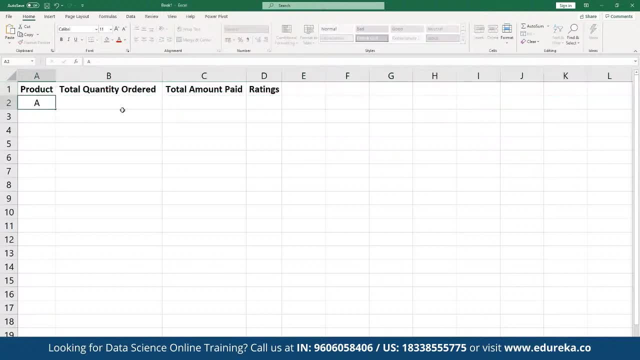 and then here we have multiple data pointers. For example, here we have product a, then we have beef, We have C, D, E, F. We have multiple products in terms of quality order. Let's say, here we have data as 55. Then we have 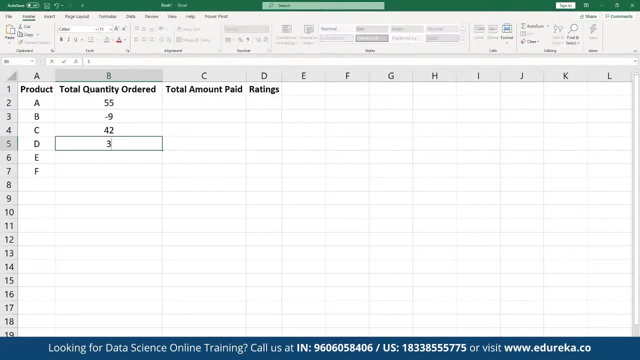 minus 9, then we have 42, then we have 35, and we have 50, and then we have, let's say, here We have a blank value in terms of amount paid. Let's say, here We have 110. here We have, suppose, say here: 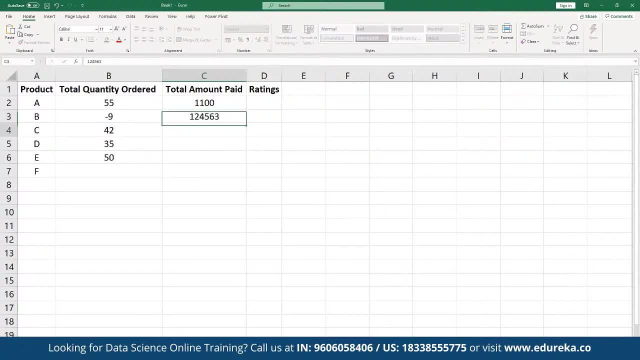 We have 1, 2, 4, 5, 6, 3. here We have 780, here We may have, let's say, 1000, or here may have a blank, or suppose Here we may have 1000 as a value being entered here. 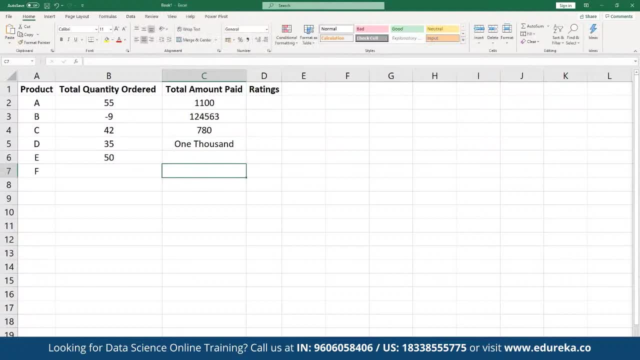 And then we may have a blank value here and suppose here we may have 800. then say me, here We have ratings, as suppose 4.2, here We may have B plus, here We may have one. here We may have minus 3 here. 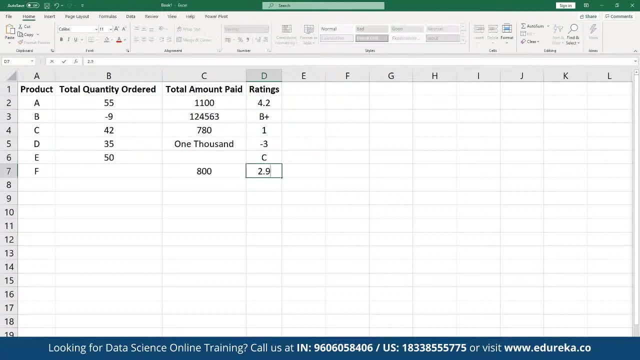 We have C and here we have 2.9.. So can we work on analyzing this data set If we have this kind of data with us along with multiple other entries in different rows, So can we analyze this kind of data set right away? 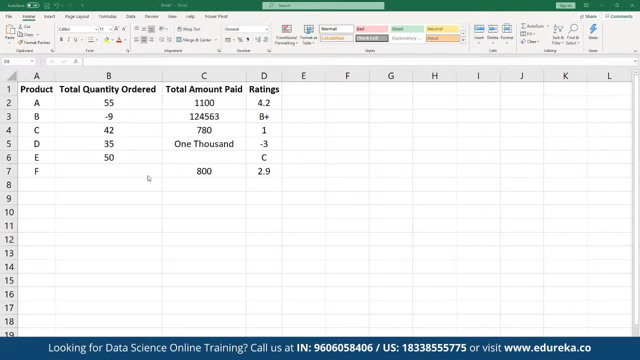 No, correct. Let's say, here we have total quality order. So if you have large amount of data sets available, so here we can define, here We can rectify the entire situation as well. So, for example, here we have the quantity in terms of 40.. 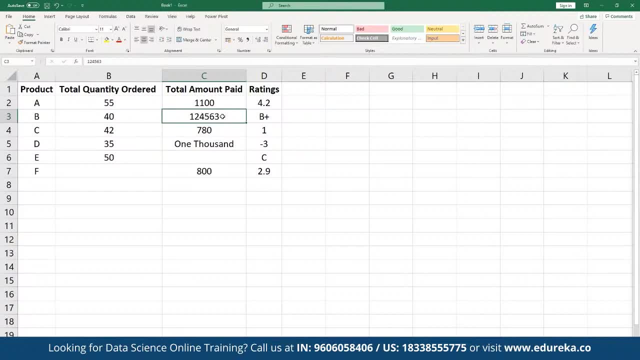 Now here it is also at an abnormal value, like we like. this is what an outlier is, so we can see how we have. major majority of the amount paid is somewhere in the range of 500, 2000 or 1200.. So one item cannot be more. 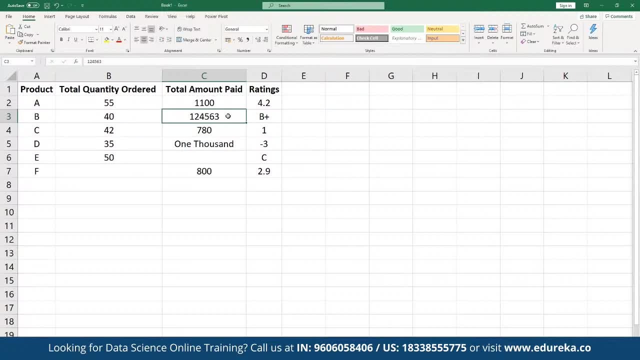 than the average value for the entire list here. So here we have a complete outlier which is towards the higher end. So again, we have to make sure we are rectifying this data set as well. for example, here we can rectify this: opposed to 1240.. 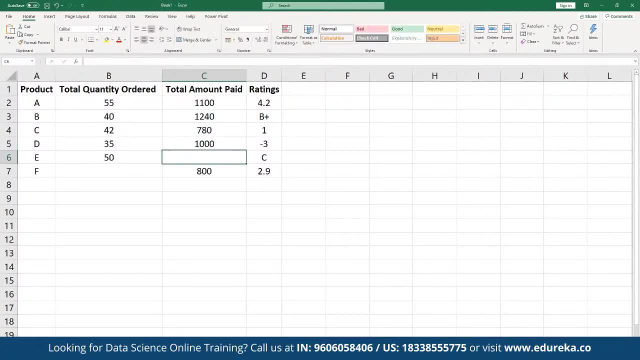 And here we have to make sure that the entire data should be in the same consistent format. There should not be any kind of anomalies there, Correct. So here we can rectify on these entire data pointers here and make sure we are having the right data set given to us. 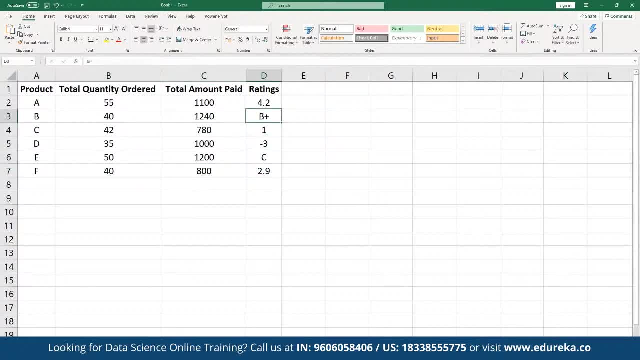 And again in terms of a of ratings. here we can ensure that we have a right rating defined for each and every product to ensure that we are not having any kind of other anomalies detector. So here we can see. let's see how we define as three. 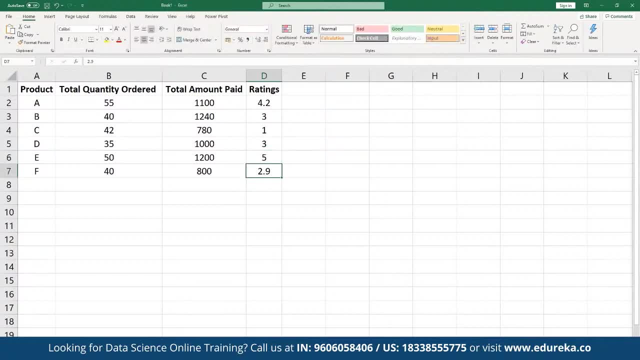 again, This one is supposed to. either they all can be in ABC format or they can be either in the same numerical format itself, Correct. So this data cleansing part, how we cleanse the data for find, by finding the average and then replacing the value there if we have multiple. 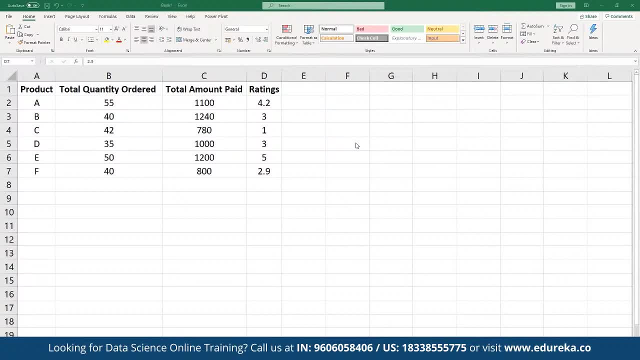 if we have small number of- for example, we have 10,000 rows available here- and if they are missing values that say only for 10 rows, 15 rows- then all we can also work on dropping those rows as well. So instead of finding the average value, the mean. 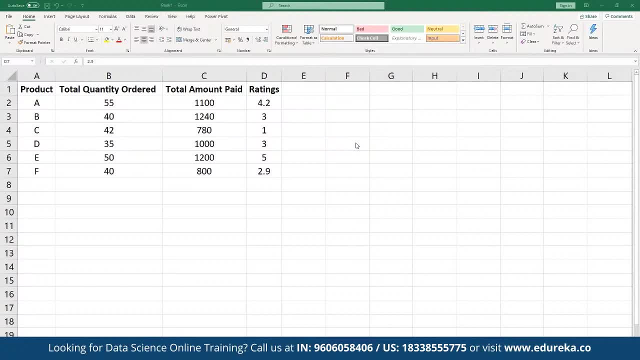 and then filling those values, so the type. so here We can find out the entire data sets here. Well, how exactly we want to proceed further? But again, this data cleansing is required. without this We won't be able to proceed further, and that's why data cleansing is an integral part. 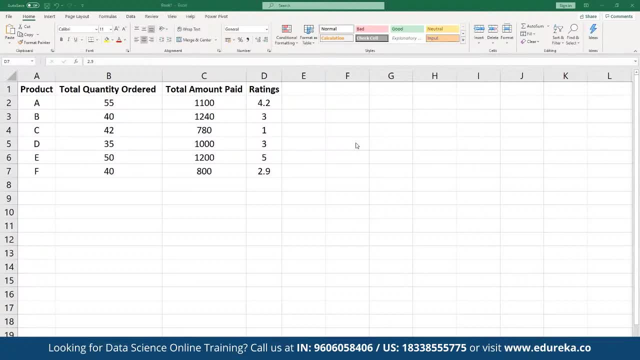 for data analysis. All right, and next we have the data manipulation part. So the process of changing data to make it more organized and easy is known as data manipulation, so that we can make use of the. so we can, for example, let's say: here we have a good or we can see. 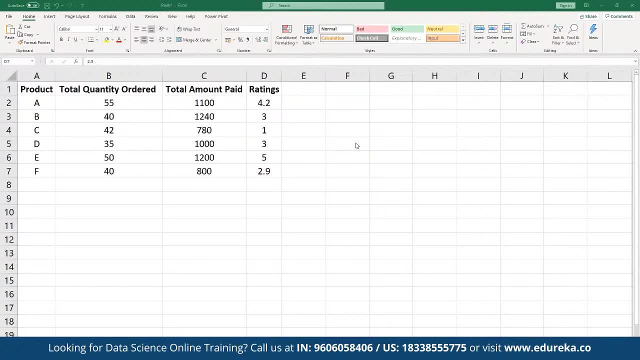 we have a good variety of data available here in different data pointers and we have large weeks, For example, we have a complete tabular, it up with us, and how we can find out the entire relationship, how we can find out the trend in a given data set. 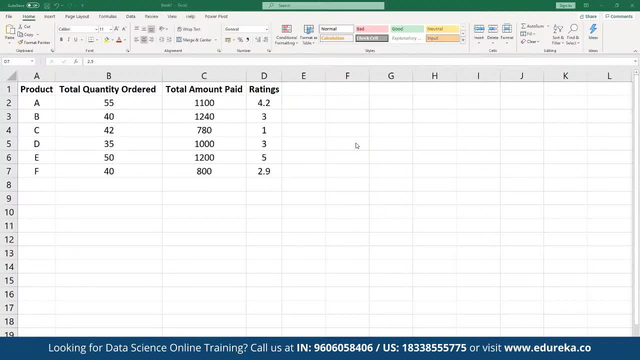 by using the right type of visualization, and that's why it is also an integral component for any data analysis work. All right, so next we have what exactly exploratory data analysis is. We have to understand this fact here. So if you talk about EDA, 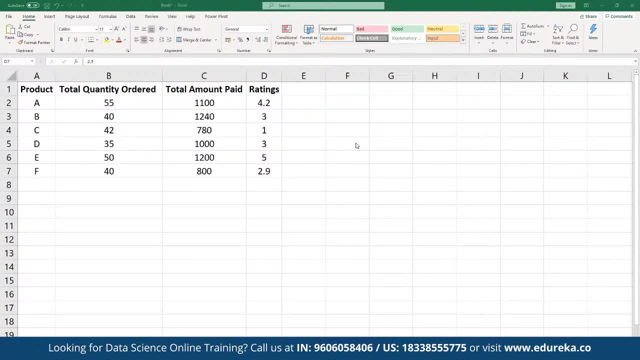 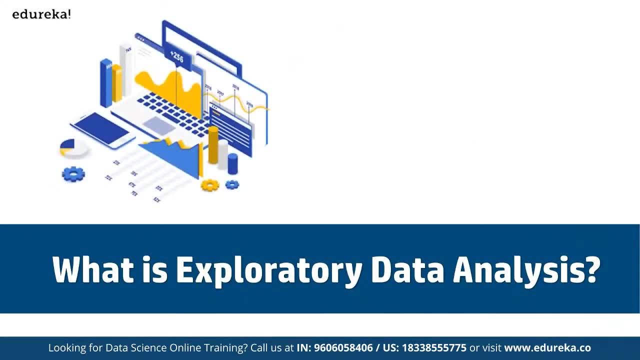 or is known as exploratory data analysis, then it is basically the first step in our data analysis process, which was developed by John Turkey in 1970.. So we can say in statistics, exploratory data analysis is an approach to analyzing data sets. to summarize the main characteristics: 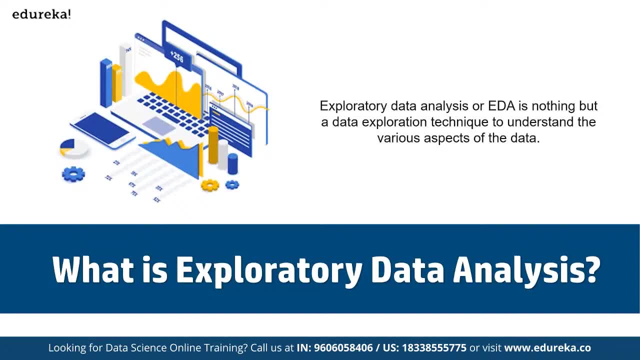 with visual methods so we can use multiple visualization methods to work on the EDA concepts. So let's say now we can take a small example here- Let's say we are planning to go on a trip to any location and things before We do, taking a decision includes you will explore the location. 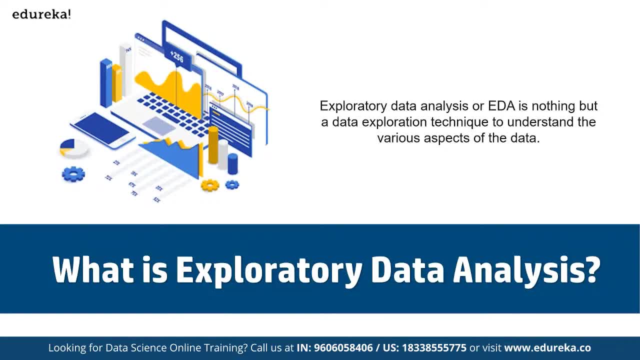 on what all places, waterfalls, trekking beaches, restaurants and location has in Google, Instagram, Facebook and other social websites. Then we are going to calculate whether it is in our budget or not and then we are going to check the time to cover all the places and then we are going to decide on the type of travel method. 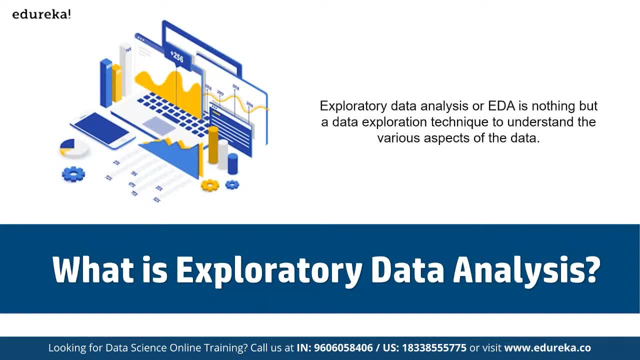 So, similarly, when we are trying to build a machine learning model, we need to be pretty sure whether our data is making sense or not. So the main aim of a straight video analysis is to obtain confidence in our data to an extent where we are ready to engage a machine learning algorithm. 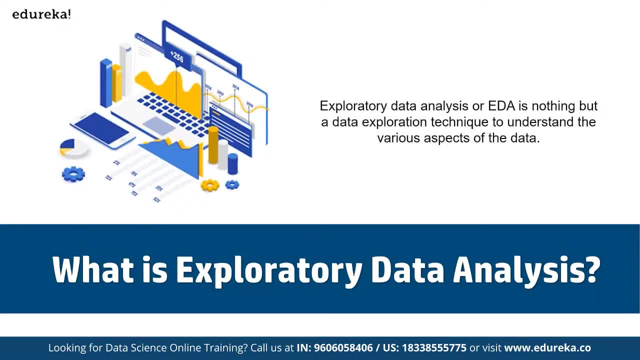 And that's why EDA is the one of the initial steps that we work on before we work on creating any machine learning models, And that's how we can say it's a crucial step before We start working on creating models to automate the system as a part of machine learning. 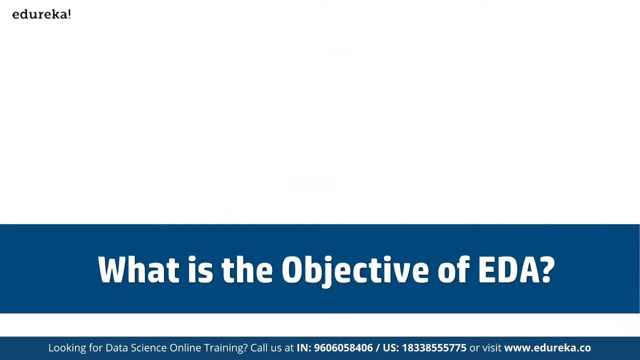 and if you talk about the entire objective here. so basically, when we are doing this now, we can get to know whether these selected features are good enough to model all the. whether all the features are required which are required is present in the current data set. 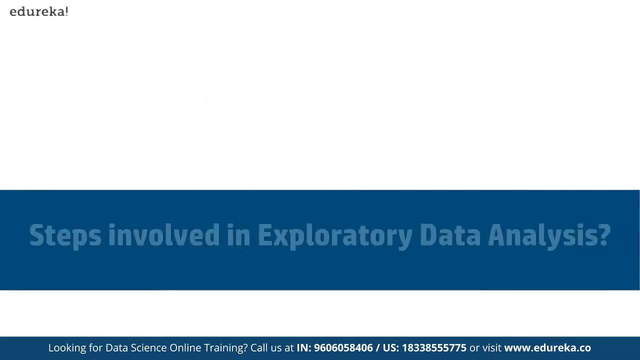 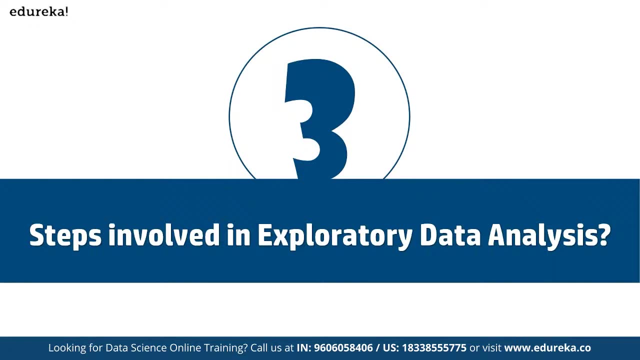 or not Right? And once EDA is complete and insights are drawn, its features are used or can. it can be used to supervise and unsupervised methods, both different types of machine learning methods. They can be used in both these scenarios here, right? 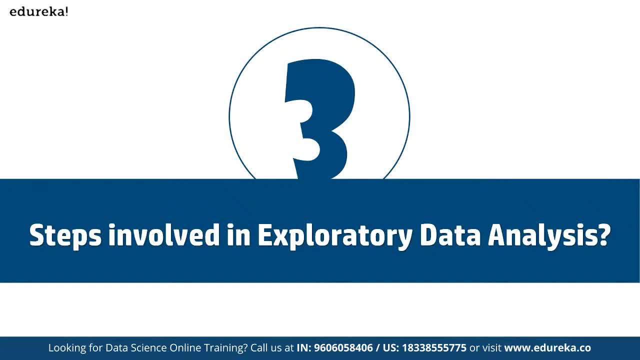 Now, if you talk about the steps involved in a straight video analysis, Before we even do that, let's say, if we talk about a simple example for EDA- let's say we have been playing a game, for example. say if we can take an example for pubg right. 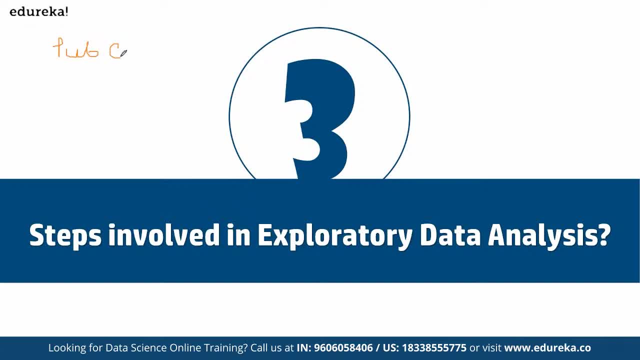 So now, when we are talking about the entire analysis on pubg, now we may have a question that does writing or can say: does killing more people ensures The winning place percentage or not? or what impact having more right distance has on the winning piece? was but winning place percentage. 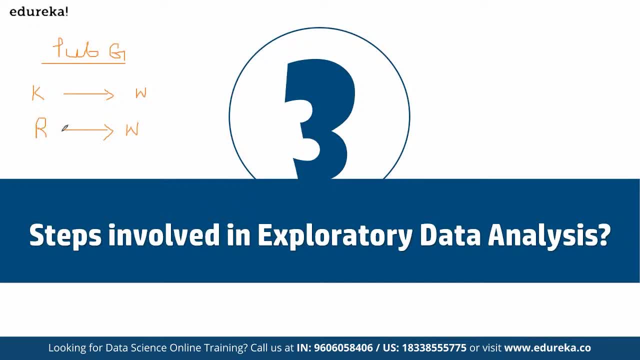 For example, if a player is able to write more than the other players, then does that mean that a player has a better chance of winning the game against as compared to others, or not? If a player is able to swim more, does it have any impact? 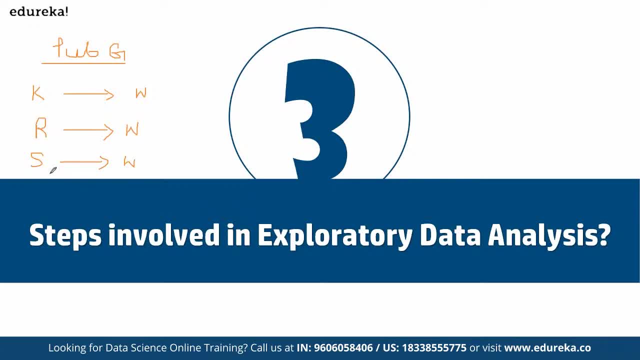 on the winning place percentage or not. That means those players who are swimming more again, whether they are having a better chance of winning the game or not. and let's say what is the impact of taking more number of heels and more number of boost items in the game? 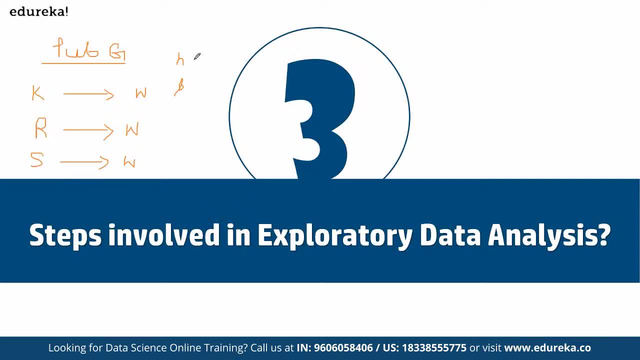 For example, we want to find out which one is going to have a better chance of winning the game- a player who has taken up more heal items, Not a player who has taken up more boost items- and not just on any random data based on the actual data given to us by the API for the game. 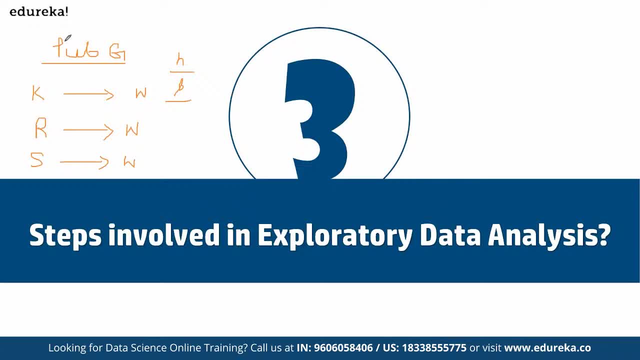 so that we can provide a solid inference that, okay, that this is what exactly is based on the given data set, whether he'll is having more impact on the winning place percentage or boost item. They have more impact on winning place percentage, right? And then we can find out the answers, both in terms 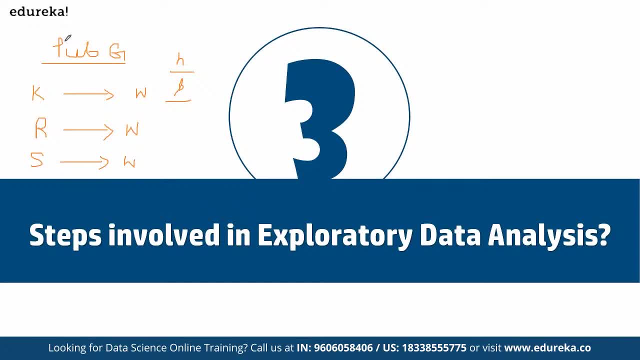 of a simple statement, or we can visualize things by using multiple visualization method. For example, we can take the data pointer for number of heat items use and then we can simply plot them by using a simple plot graph and then we can compare these two different plot graphs. 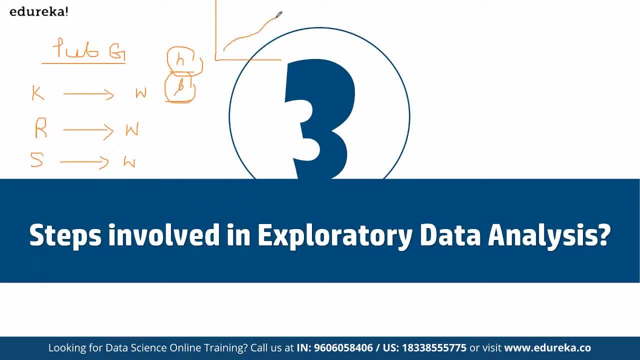 to see which one is have a bitch one is more closely related to the winning place percentage, correct? So the this exactly is what EDA, or we can say x-rated data Alice's, is used for for finding, So for making sure that all the hypothesis. 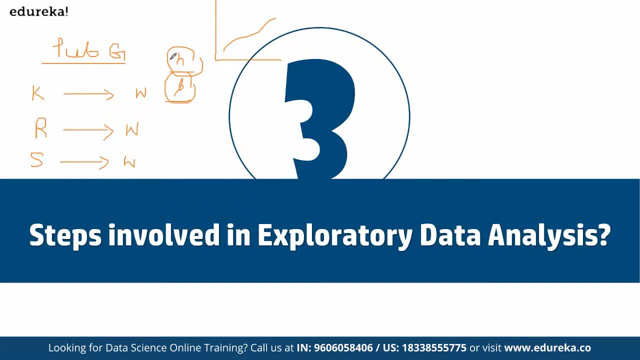 that we have for any wrong statement. they are true or not. All right, so let's proceed further Now. if you talk about the steps involved in EDA, then there are multiple steps involved here. First of all, we have to understand data. 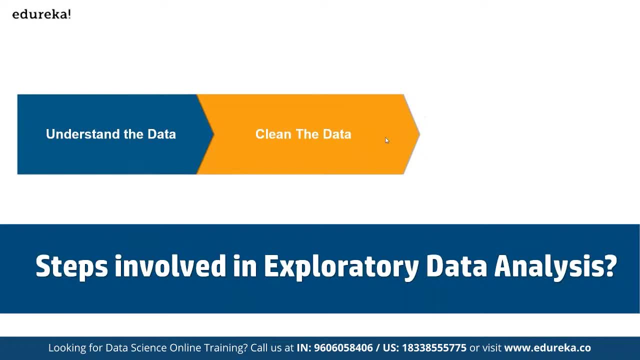 Let me what, exactly what kind of data we do have the access to. then we have to work on cleaning the data and then we have to work on setting up the relationship between different variables and we can use it for a better understanding how the relationships and new insights are defined through plots. 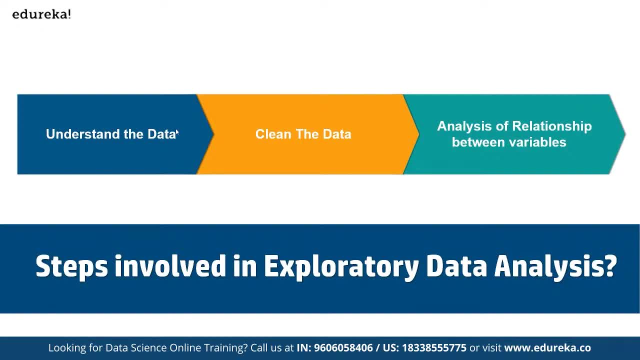 So, first of all, if you talk about understanding the data, so we need to know the different kind of data and other statistics of our data before we move on to other steps are good way to start with by using the describe function in python That we are going to look at in next few minutes. 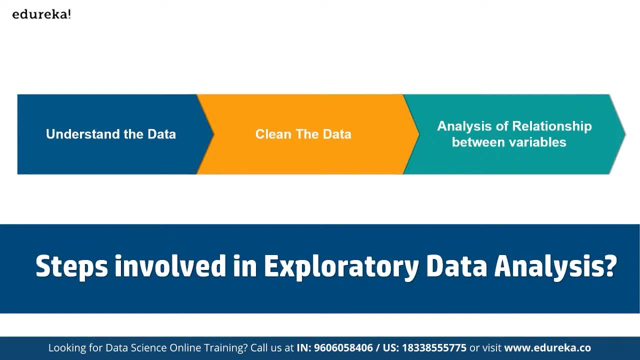 and then in pandas, which we use for creating multiple data frames. It's a library so we can apply, describe methods on a given data frame, which helps in generating descriptive statistics. that summarizes a central tendency, dispersion and shape of a data set distribution, excluding the null values. 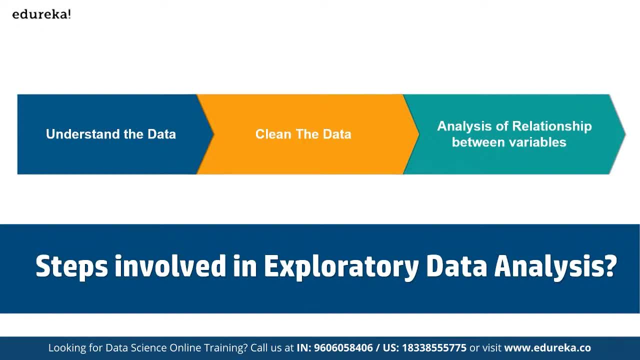 So to start working on a simple data analysis job, so we can take the head, we can take help of any Sample situations here. So we are going to take the. we are going to take the help of analyzing a simple problem statement by using a game such as pubg. 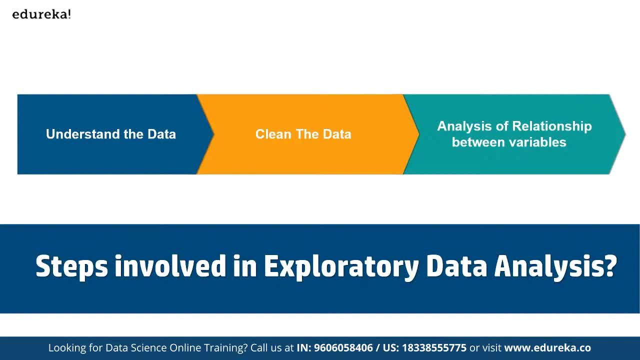 So we already have a notebook defined, So we're in this notebook, We are going to work on such analysis. So let's do one thing: Let's fetch that particular example Here for seeing how the idea concept works, so that we can have a better understanding. rather, 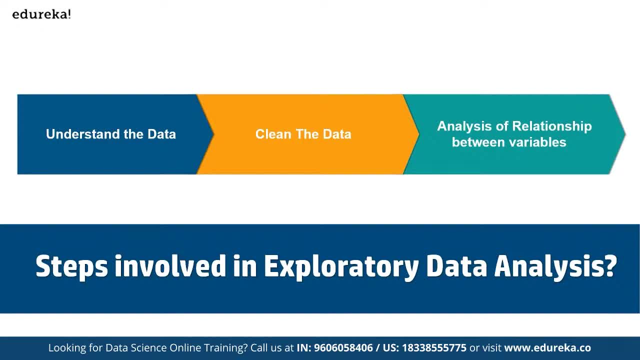 than just to talk about it. So we have discussed: give us a fall. We have to make sure we are able to understand it in a much better way and we have to work on cleansing the data so that we can remove any kind of anomalies, which includes outliers and normal values. 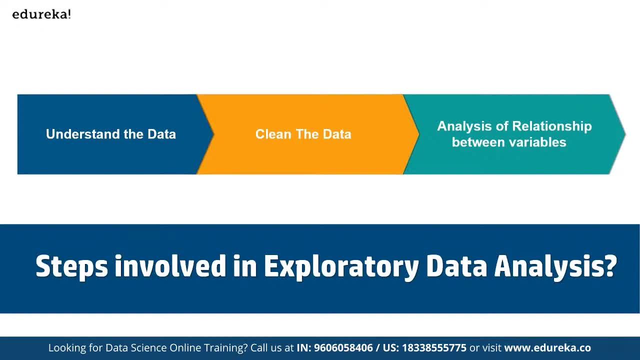 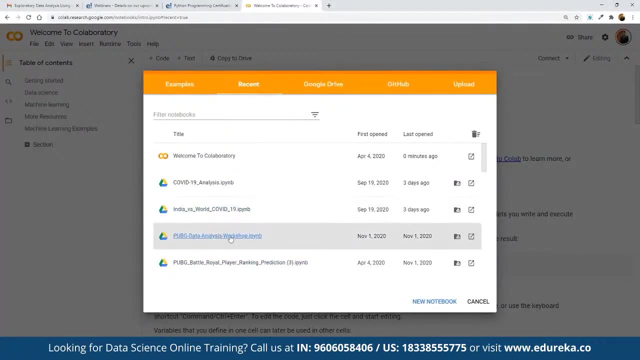 and then we had to work on setting up the relationship. That means you can work on finding the correlation of multiple data pointers together. So here in ETA, So here we are going to make use of this pubg data analysis. So here we are going to make use of this entire analysis. 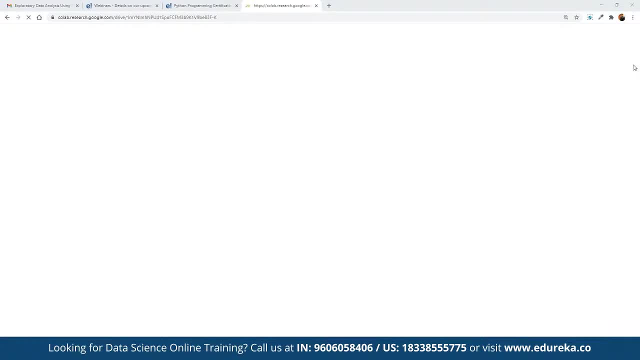 file of this net, that notebook file, to see how we can find out multiple, how we can validate multiple hypothesis on this game. So we are going to find out how we can work on cleansing the data and as well as how we can work on performing multiple ETAs. 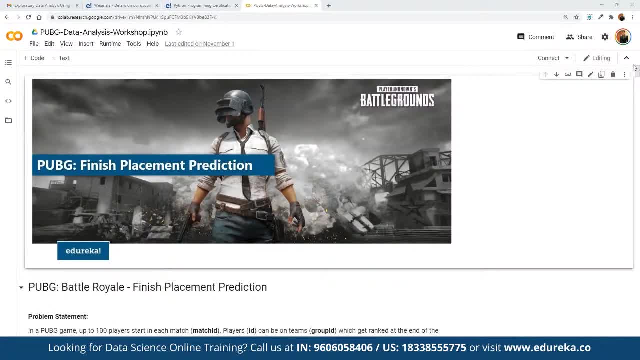 to validate multiple theories on this game. So now to see how exactly ETA works. We are going to use python for performing this ETA, So here we are going to work on the pond. performing the ETA consists on pubg game. So pubg, as we know, is one. 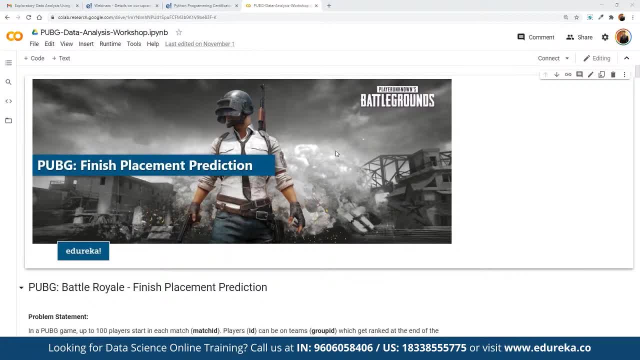 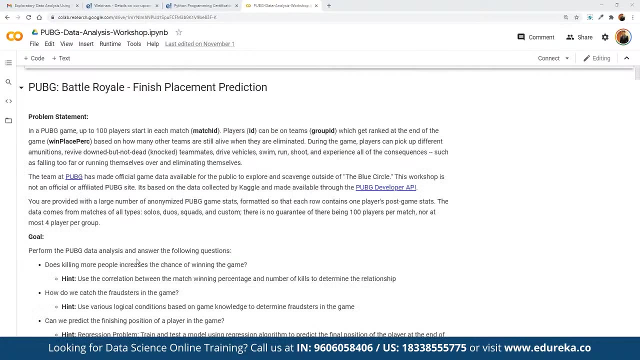 of the most popular multiplayer game in the world and to start working on the ETA concepts, For example. the premium main problem statement that we are going to work on is to find the answers to these most popular questions, like we have. thus, killing more people increases the chance. 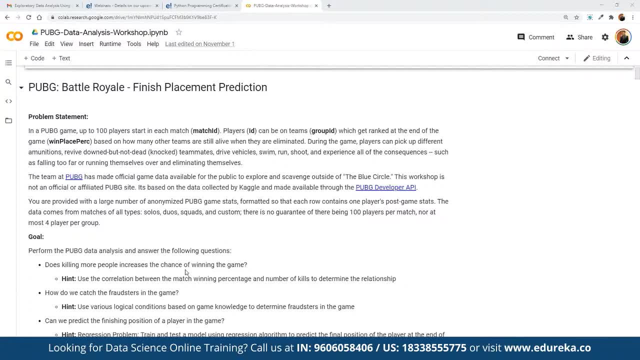 of varying the game. So again, it is also a concept of ETA. So here we have to find the correlation between a match, meaning match, winning, place percentage, along with the number of kills to determine the relationship, And then we are going to find out how we can catch the fraudsters. 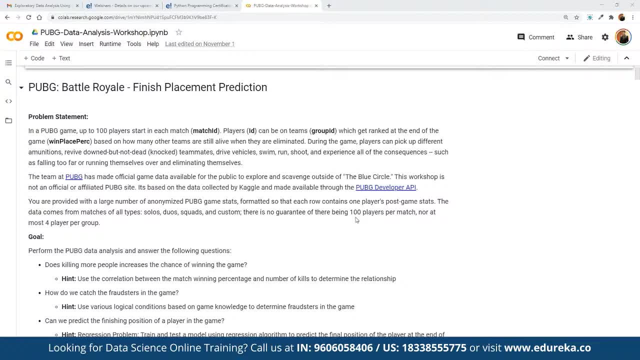 in the game that when we talk about fraudster, that means we are going to find out multiple app. We can say outliers. That means we are going to find out the values, which, again, we are going to find out the players who may have used multiple kinds of cheats. 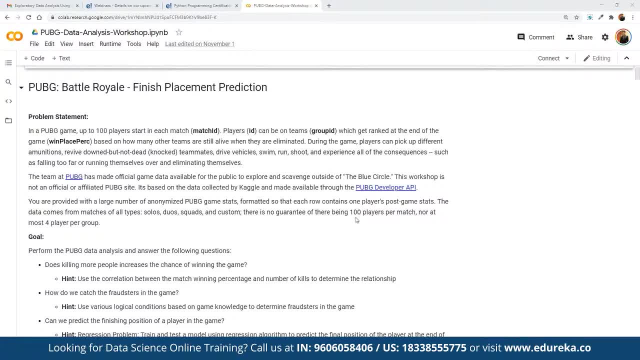 or multiple kinds of aimbots. So we have to remove that data and then we can work on creating a prediction model as well. So we know that pubg is one of the most popular multiplayer games, where we can play in three type of matches. 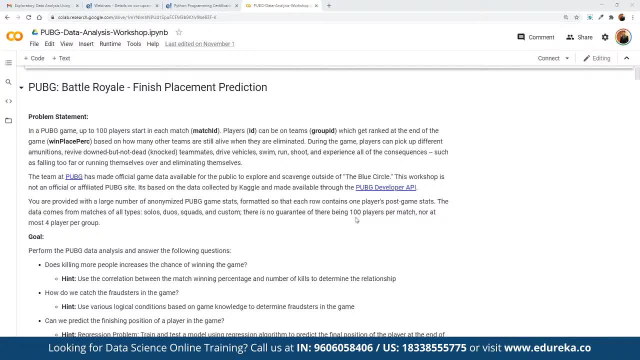 We can play either a solo, we can play with two players, or we can play with later squad of four different Players. so to find out the answers to these different questions, First of all we have to understand the data set. So for that we have to make sure we are having a complete data available. 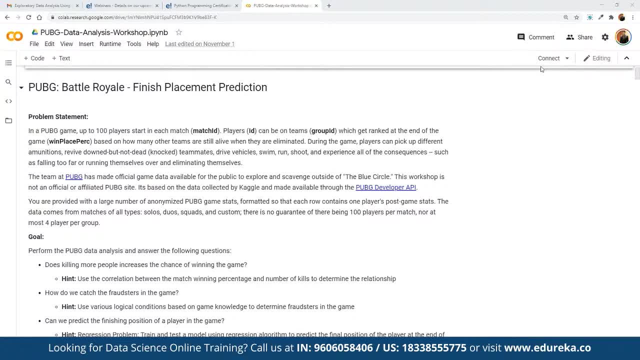 with us so that we can start performing the analysis. and here data is already available by PUBG itself by its official API. So PUBG has made 65,000 data for its 65,000 matches available on kegel, So we can use this data set to get started on the actual analysis. 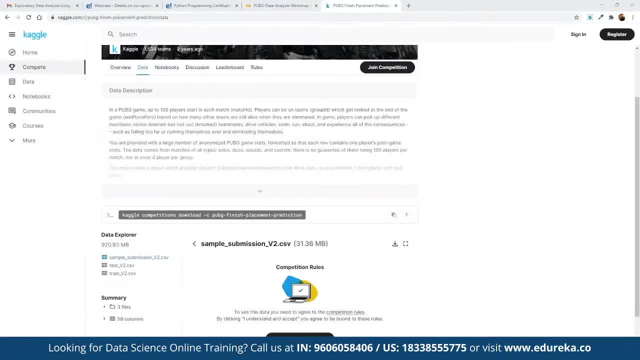 So here we can navigate to this link here from kegels and here we can find out the actual data set. Now This is the actual official data set available. There's no sample data, So this is not a sample data or any random data set. 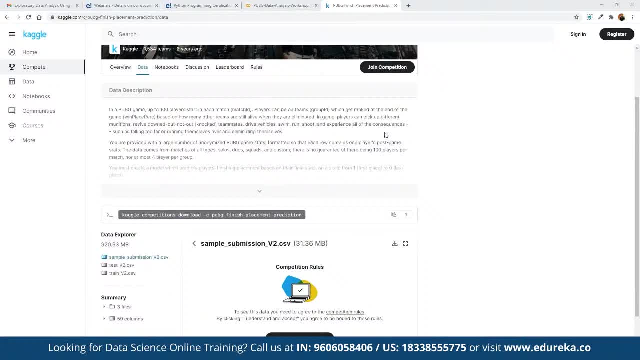 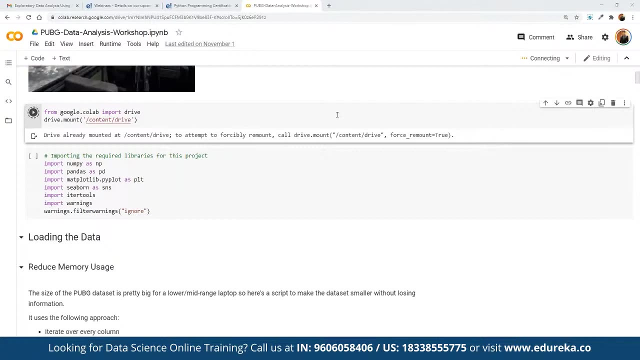 This is the actual data set available that we can perform the entire EDA on. Now we can come back. So now, before we can get started, we had to Mount the Google Drive where we already have uploaded the current data set. So, if you want, we can also work on Jupiter as well. 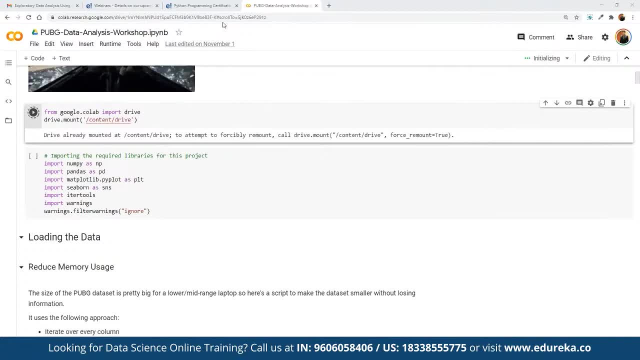 We can work on Jupiter notebook, or we can work on the school app given to us by Google. So once we have downloaded the data set from the link that I have shared with you all, we have to upload that data in our Google Drive and then we can Mount Google Drive with collapse. 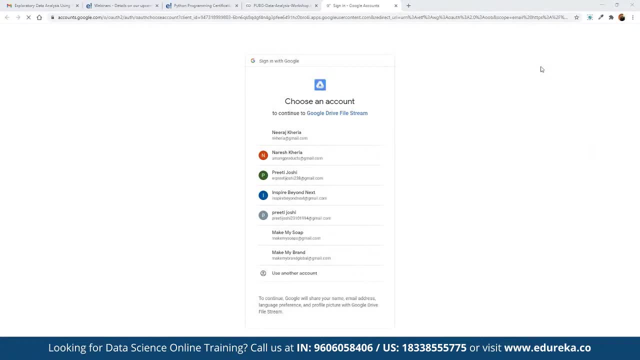 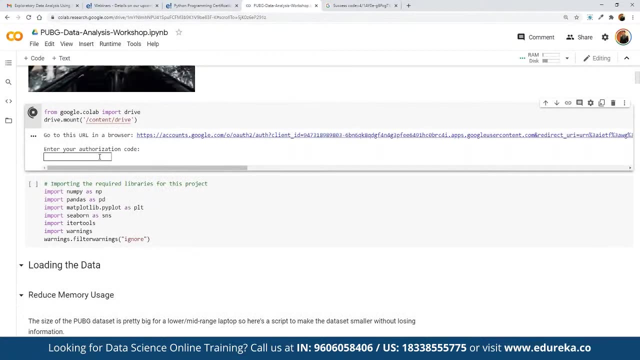 so that we can get started. So we have to Mount it first. So here we can mount It. so once we use from Google Colab, import right and then we can specify the location of Drive and then we will be given an authorization link. 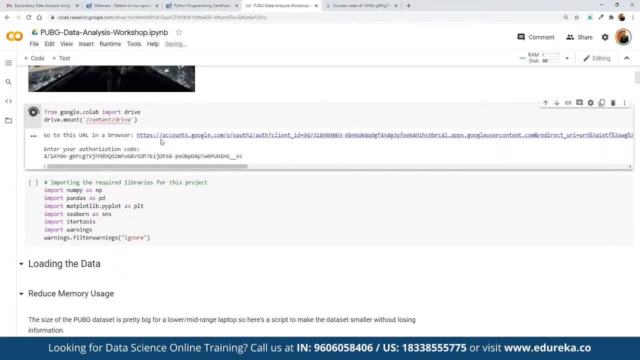 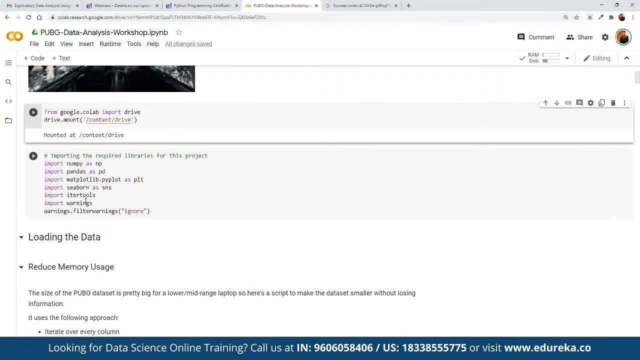 So once we authorize this, with the account on which which we have uploaded the entire data set and we can start working on it. So now we are going to work on these libraries. So we have, we are going to import number for the calculation pandas for creating multiple data frames. 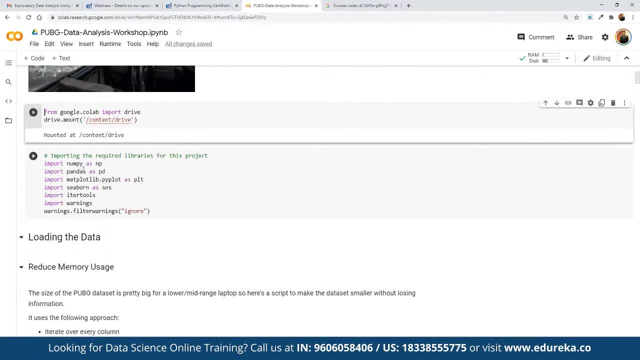 Then we are going to use matplotlib and seaborn for the visualization. matplotlib is used for small data sets and we have large data set and we want to make use of advanced visualizations. Then where we you make use of seaborn library and then for performing iterations. 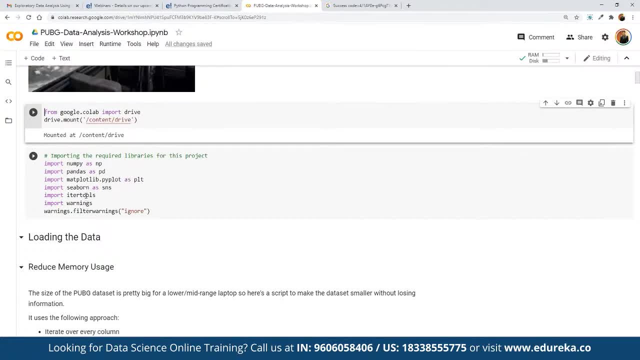 We are going to work on iteration tools And then we are going to ignore warnings by importing the warnings that may be generated for multiple data pointers that we are going to use here. Now, once we have the libraries imported here, then we are going to read the files. 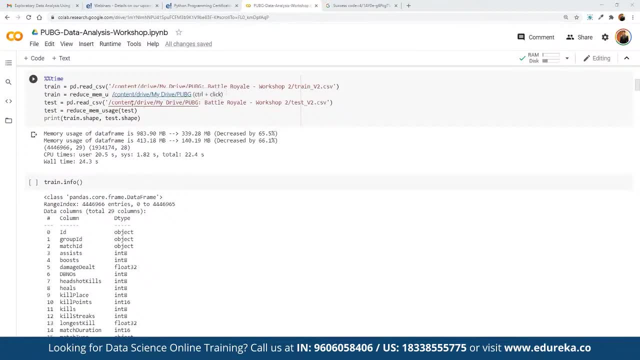 which has already been uploaded in our drive. So we bought reading the files. here We are going to make use of PD, as in pandas, and then we can Define the read function, the read CSE function defined under pandas itself. So here we have to Define the path where we have see the file. 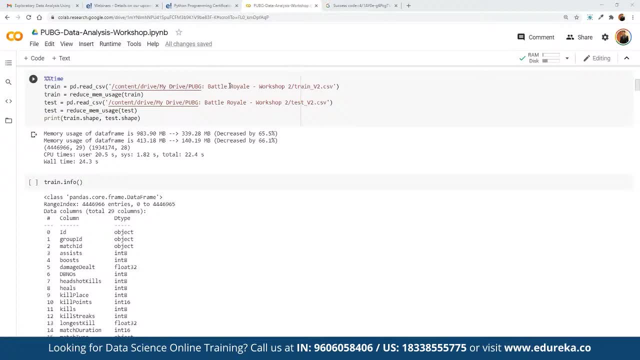 So we already have a file uploaded in a drive and it's under the folder of pubg- battle Royale. And same way, we are going to import both of these data set. We are going to import the test and training data set, for example, when we are working on creating a prediction model. 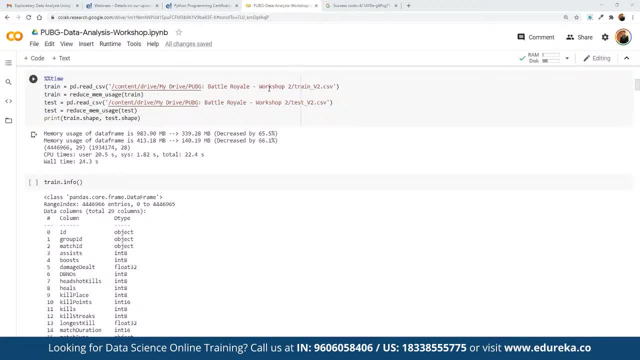 so we generally split the entire data set. We split the entire data into equal parts. We split them in training and testing data set So we can create multiple split. So, for example, let's say when we are working on training any systems and then we don't train the system with all the data pointers. 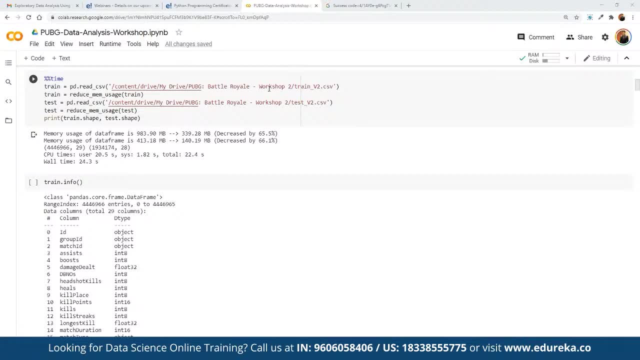 because if you use The entire set then they will be nothing left to test. great, So we use 75 to 80 percent of data to test, to train, and then we use the remaining remaining 25 to 20 to 30 percent of data for testing that project. 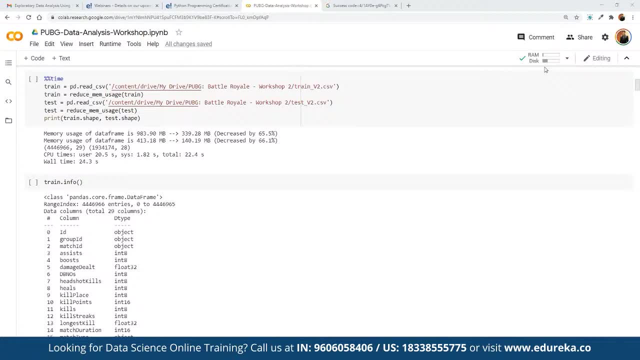 And then to find out now, once we are done fetching this data from these different data sources here, so we can simply find out the entire information that we want. So once we have loaded the entire data set here, then we are going to simply execute it and then we will be able to find the data uploaded here. 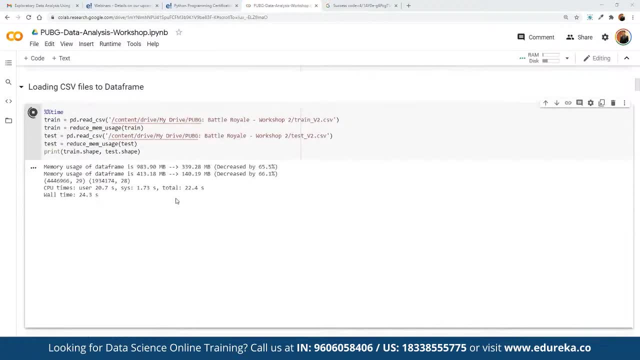 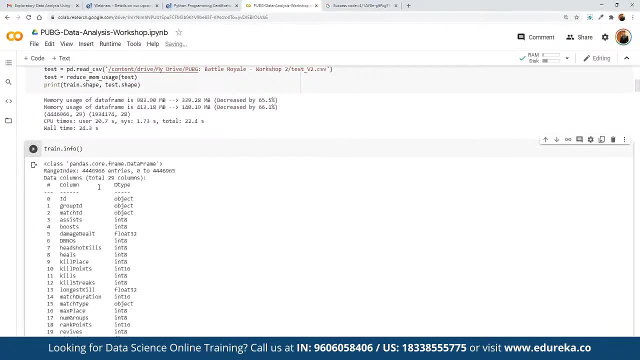 So here we are going to simply fetch. as you can see, our data is currently being fetched. Run the given data frame here and now to find out the information about the current data. you can use trained or info, and then we can see the list of all the columns. 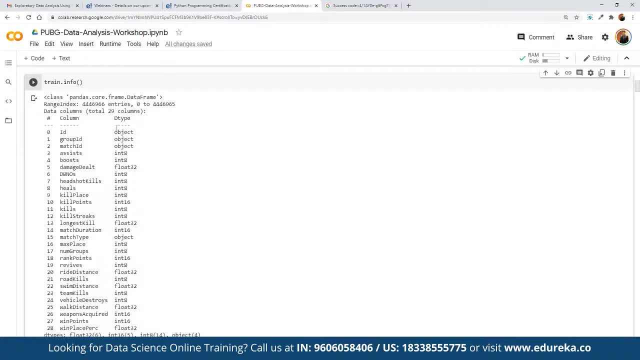 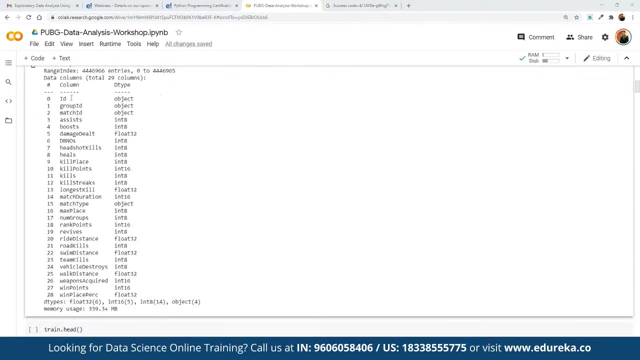 that we have, along with the data type, stored in these data sets. Now we can proceed further. So we have multiple data points Here. so we can see we have data pointers such as the group ID. So ID refers to the exact user, then group ID refers to group. 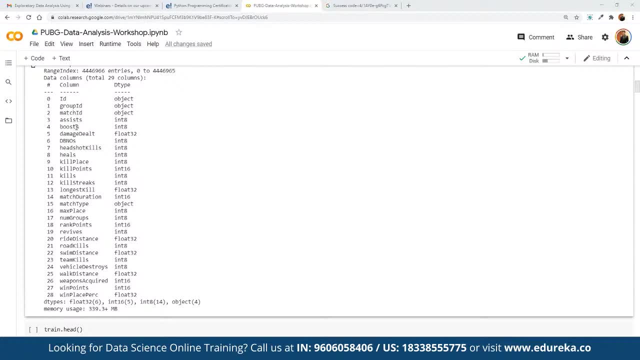 and then we have match ID available. So we have- the number of us is taken up by the users- the number of boost items, the number of knockouts, the number of kill plays, number of headshot kills, the kill Streaks, as per the requirement. 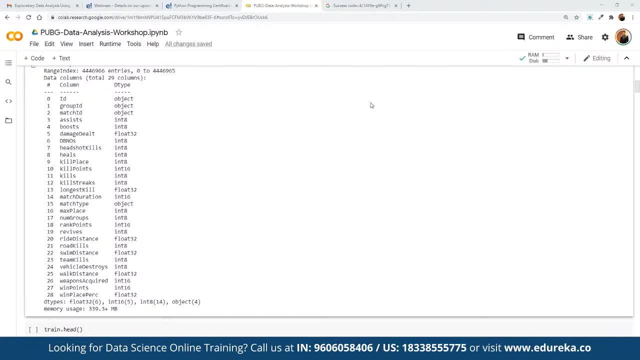 All right. so now to work on the actual area here. So now we can start working on multiple exploratory data analysis components Here we are going to work on the actual experience. We can say exploratory data analysis here. So let's say the first thing that we want to analyze: we want: 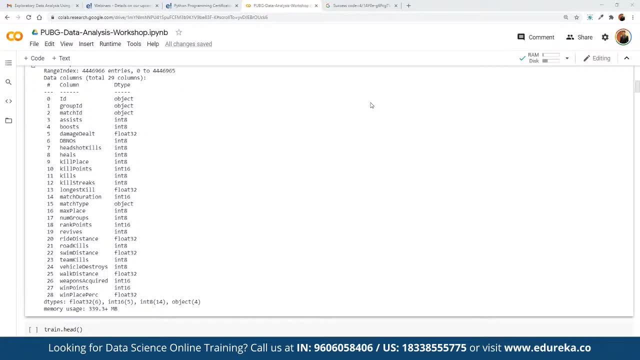 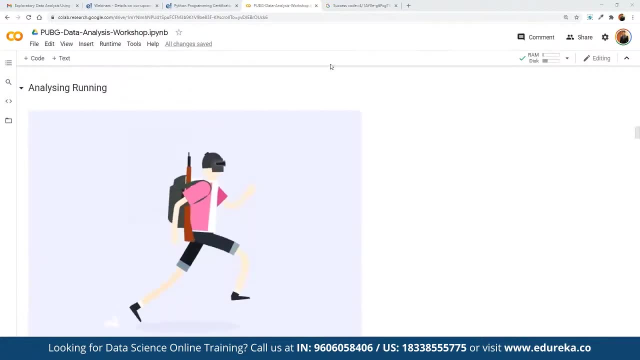 to analyze the effect of heels and boost items. We want to analyze the effects of running as well. So first of all, let's say, as a part of our EDA, We want to analyze running. what impact running has on the winning place percentage? 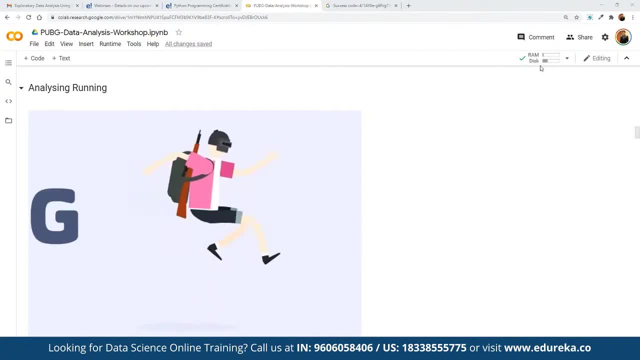 That is what we want to analyze here: What is the impact running has on the winning place percentage here, and for that we are to first of all make sure that we are running a statement. now we are going to make use of python, correct. 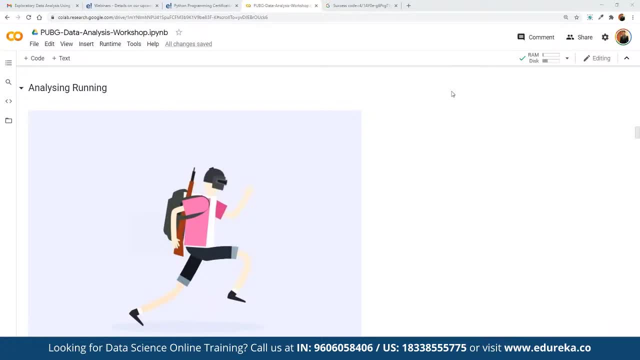 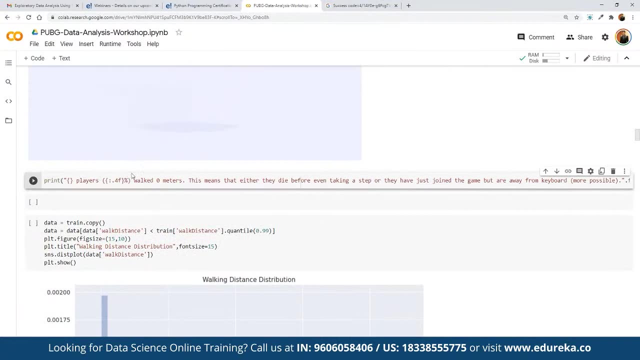 So when we are going to make use of python, we can define the entire python line here. For example, let's say: here we want to find out The number of players walked. are how many players they have walked for zero meters And this means there that they die even before taking. 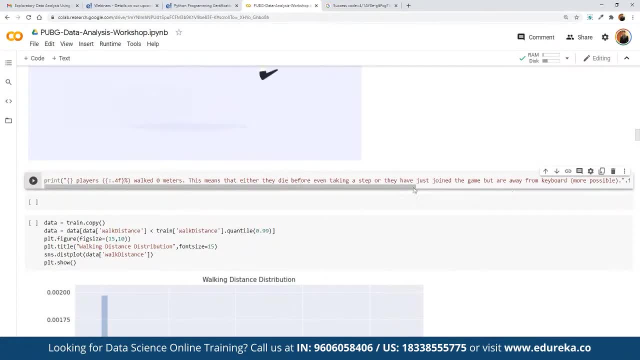 the first step, or they have just joined the game, but now they are away from the keyboard. So how many players are there which fall where? who falls into this category? So for that, we are going to simply define a statement where the walk distance is going to be zero. 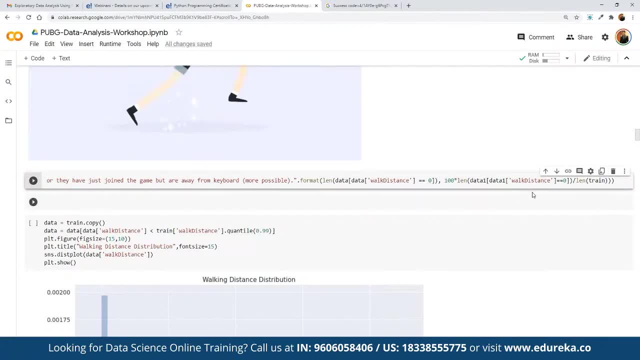 from the current data frame that we have created, and then we are going to find out the walking distance, again in zero, based on the data pointer. So again, then we are going to simply divided with the training data set. So if you run the statement, 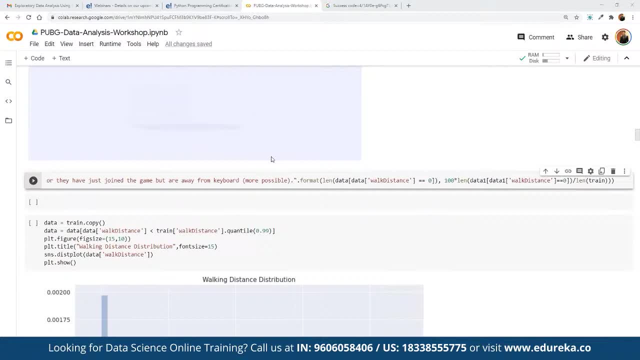 we will be able to find out the number of actual players who are who fall into this category. same way, if you want to find out the effect of healing and boost items, for example, suppose if you want to find out the effect of riding on the winning place percentage. 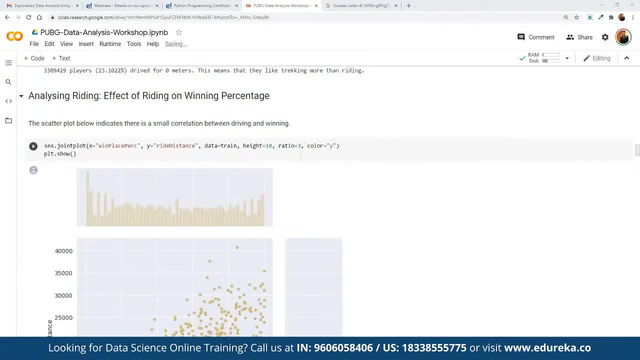 then we are going to make use of SNS library as an seaborn library, where we are going to make use of joint plot, where on x-axis we can place very increased percentage and on y-axis we can place Right distance, and then, by using the and then we can find data to be origin. 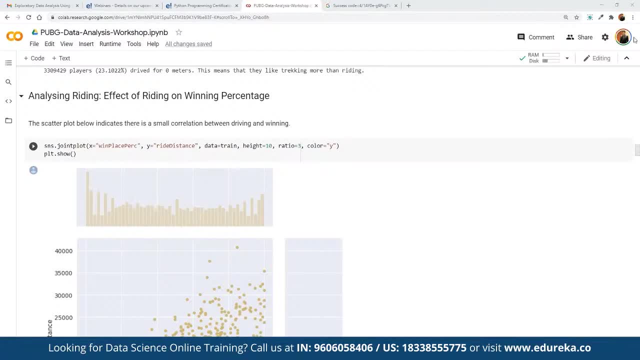 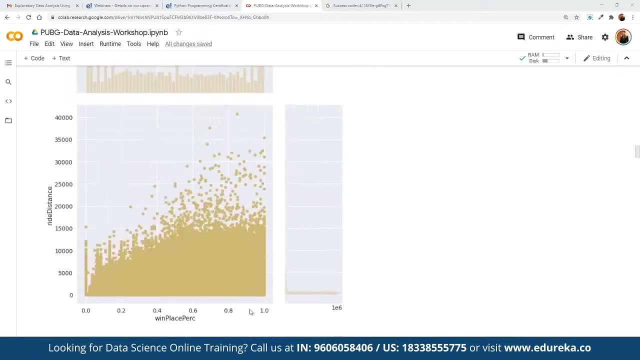 data to be used for training and if we run a statement and we will be able to see this kind of graph being generated here, So where we can see the actual effect. that means on x-axis We have the wedding place percentage and on y-axis we have the right distance. 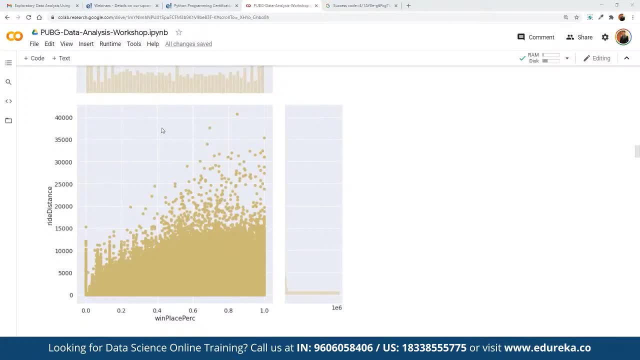 So here we can see: as the right distance increases, So does the wedding place percentage as well. So here we can see how what impact it has, As on the ring place percentage, as with the current definition defined. So now we can infer from this current diagram: 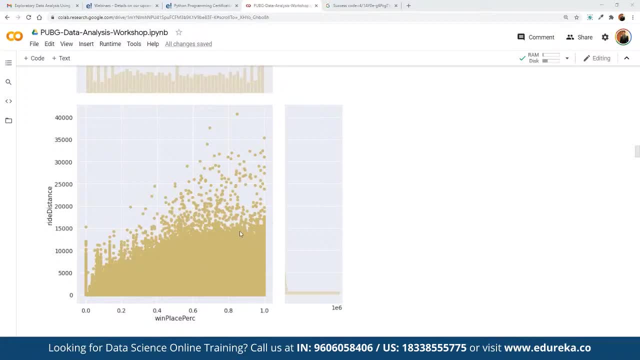 So, theoretically, if a player is able- not here- we can simply infer so again, we get simply infer that. okay, if this is the case, that if the person is able to write more in the game, then the person is going to have a better chance of winning the game. 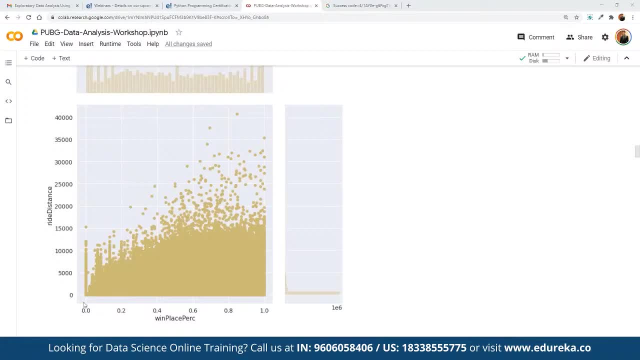 because, in terms of correlation and the value is closer to 0, that means it has no impact or it has no impact at all On the winning place percentage and the value is going to be closer than 1 to 1.. That means the chances of that means this value is going to be highly correlated. 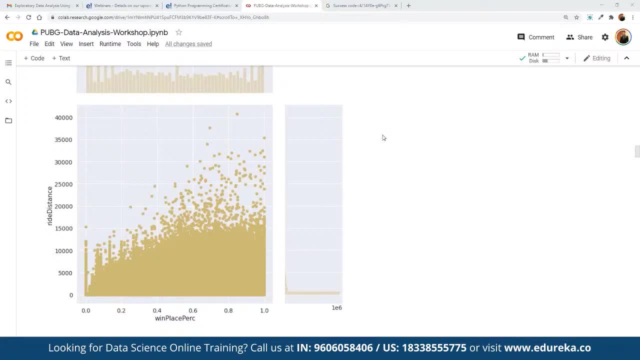 with the other value defined here as a part of correlation. All right, and as we discussed again when we are working on this analysis, we also need to do the entire cleansing as well And to work on again same way. We can also find the effect of healing. 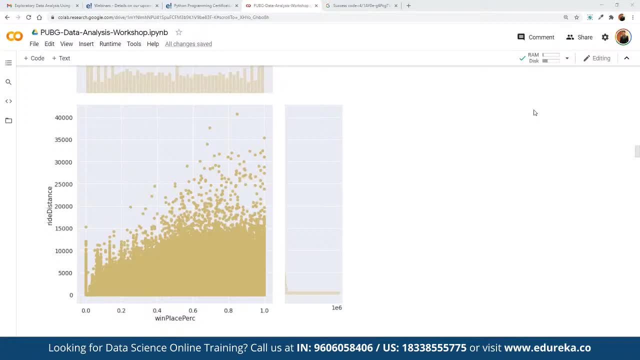 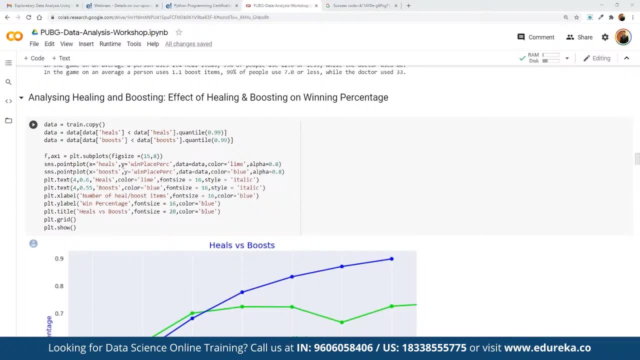 and boosting on winning place Percentage. So let's say, if you want to find out the eating without meaning here, so we can simply use a point plot graph here. So again, here we are going to find out. here We are going to simply plot the effect of heels. 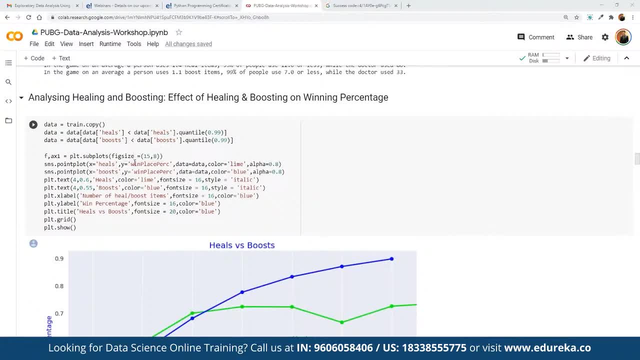 So on heels, we are going to plot on x-axis and on y-axis We are going to plot the winning place percentage. same way, in the same point plot graph, We are going to plot the boost on x-axis and on why we are going to place winning place percentage. 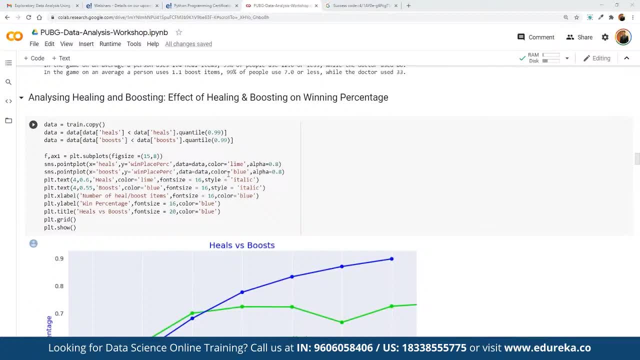 and then we are going to give them a different color and then we are going to define The labels, their colors and their percentage. And if you see the current diagram here, we can see the impact of heels versus boost. So we can see both of them. 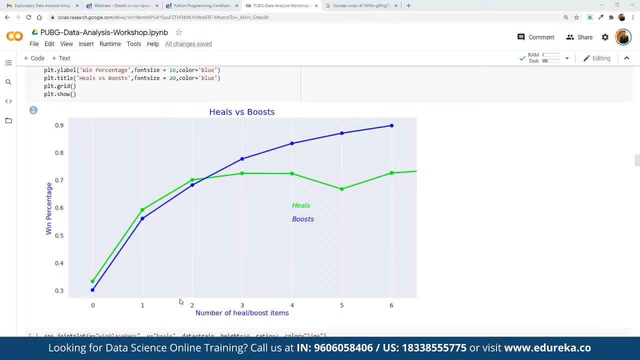 They have a high correlation with the winning place percentage. But as you can see here, if the number beyond the two boost items or two heel items, the beyond two heels, again, the curve here simply Flattens right, So it doesn't have that high impact. 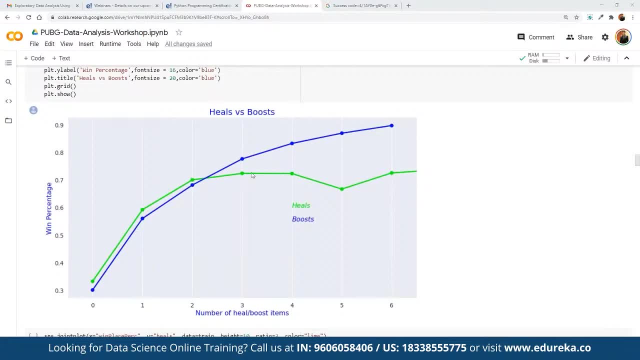 on the very increased percentage as compared to the boost items. right. So here we can simply get now. here We can simply infer that again, Both of them have a high correlation with the winning place percentage, But again, boost is going to have a better correlation. 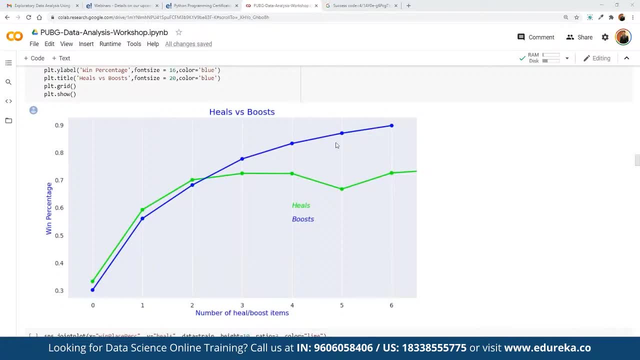 That means if a player is able to use more boost items, then the winning place percentage of that player is going to be better as compared to those who are going to take more number of heels as compared to boost items. So these are the simple. 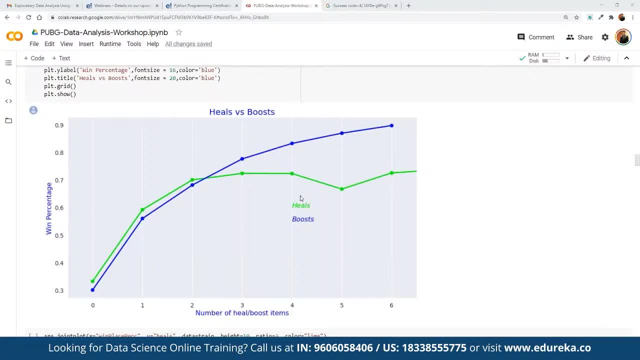 Again, what exactly we are doing. We are simply testing our theories and we are simply seeing the actual father, whether this theory stands true or not, by using multiple ETA concepts. And same way, We also have to work on multiple data cleansing method as well. 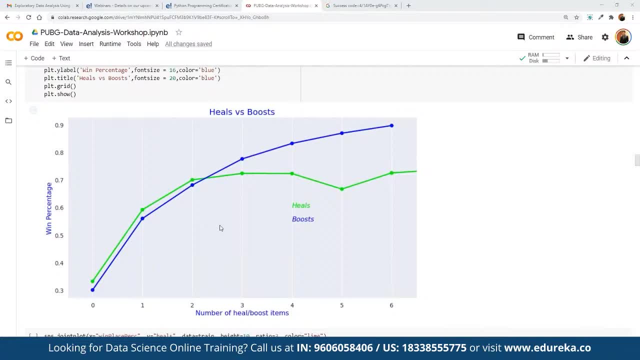 where we can work on removing the outliers. So simple example. let me show you a simple example for removing the outliers. or we can see how we can work with data cleaning methods. So first of all, we have to make sure we are We are removing all. the record says: 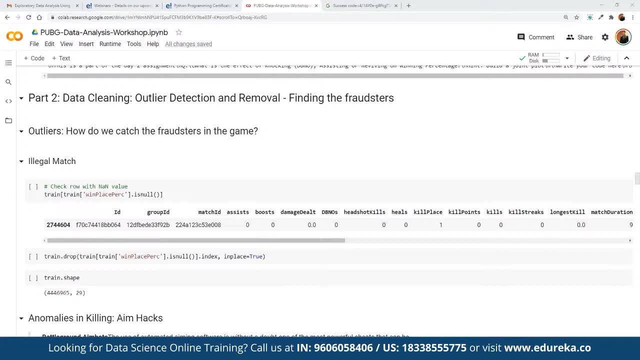 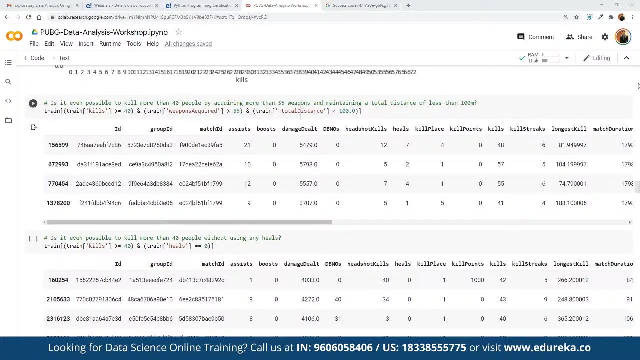 which are having abnormal values. For example, we have someone- Hannah, someone may have in human skills have again say so we can find out those, God say, against those data set in a given data. So let's say, if we have this kind of of question, 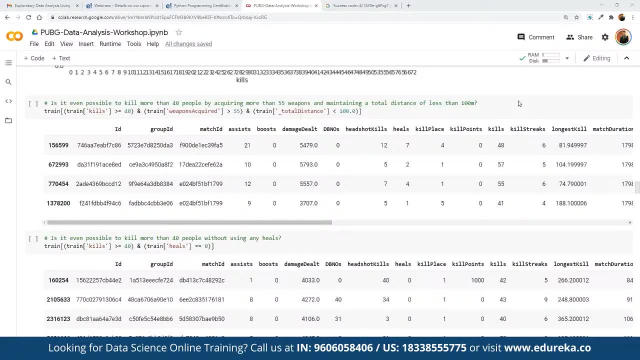 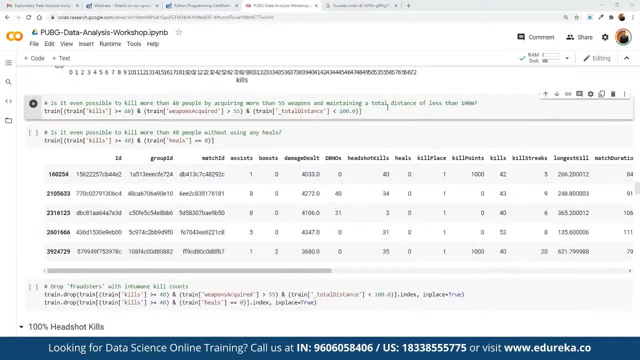 for example, here we have a statement: Is it possible to even kill more than 40 people and by acquiring more than 55 weapons and maintaining a total distance of less than 100 meter? So for those who have been avid player of this game, 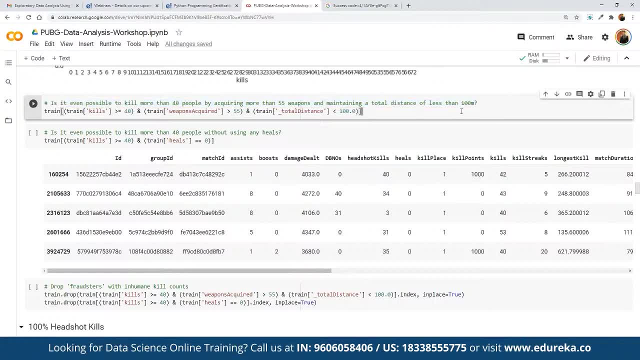 place of this game. So is it possible everyone To kill more than 40 people by acquiring more than 55 weapons and maintaining a total distance of less than 100 meter? Is that practically possible? We know it is not practically possible, Correct? 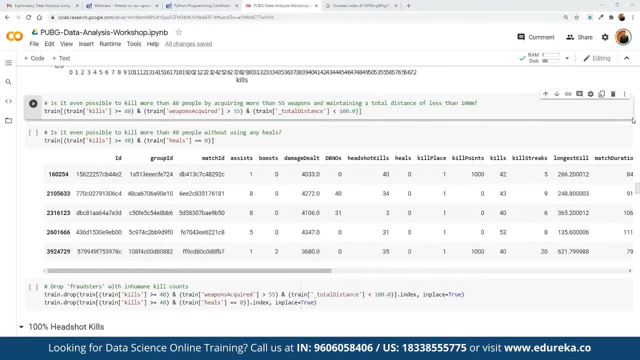 So we have to make sure that we are removing now again, if we include these data pointers, that means obviously they are going to be outliers and they are going to impact the actual Probability credit and that's how we have to make sure we are removing these kind. 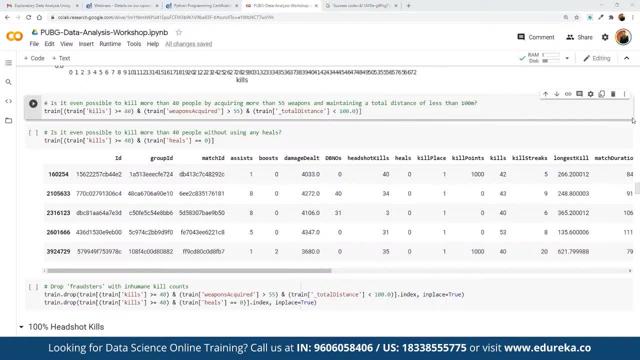 of our tires, So that we can improvise the accuracy of the model that we are going to create here, Correct And, let's say, if we run the statement here, we will be able to find out the exact number of people who have who fall into this entire category: cells. 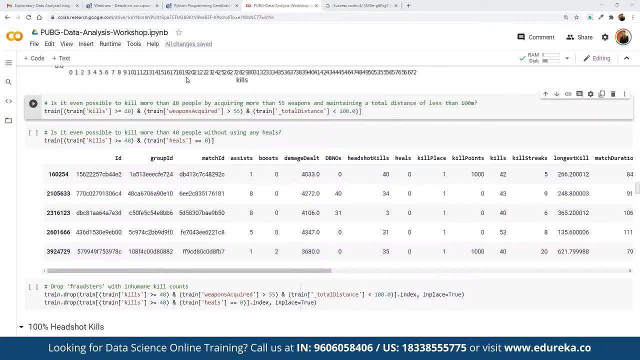 So here we can see next same way. If you want to see, to find out, Okay is it is been possible to kill more than 40 people without using any heels? Then again, we are proud. We know practically this is not going to be possible. 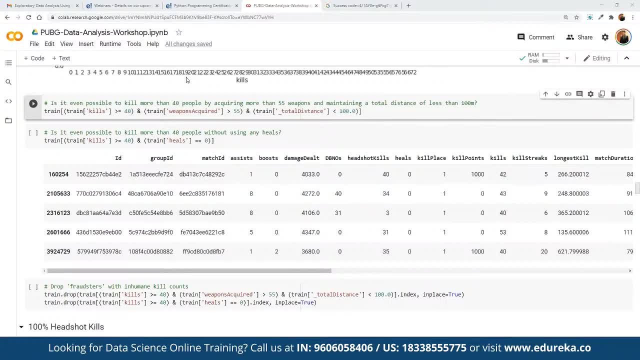 So we have again. We have multiple data pointers to help us out with and, as a component of EDA, as an x-ray tree data analysis here. Same way, We have multiple other outliers As well. So, for example, here we have the headshot kills. 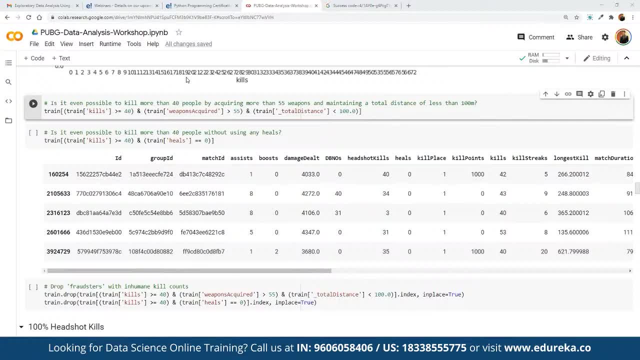 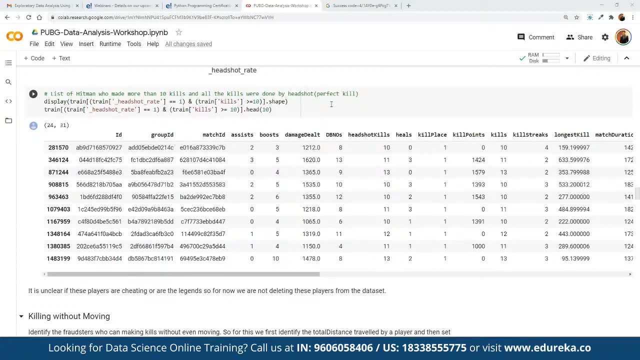 So now we want to find out the list of all the Hitman's available here. So let's say, here We want to find out the Hitman who has made more than 10 kills, and all the kills were done by headshot. So we know again that this can be done either by two people. 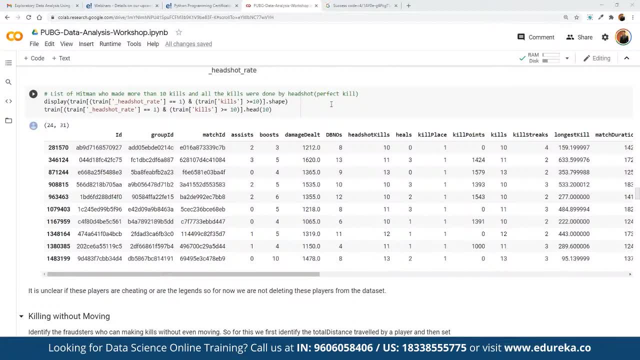 like we, either the Hitman hits is in self or by John wick, or else they will be released called as a skill personnel for having this high amount of kill rate. So for finding out Those players who are having every, who has every kill done. 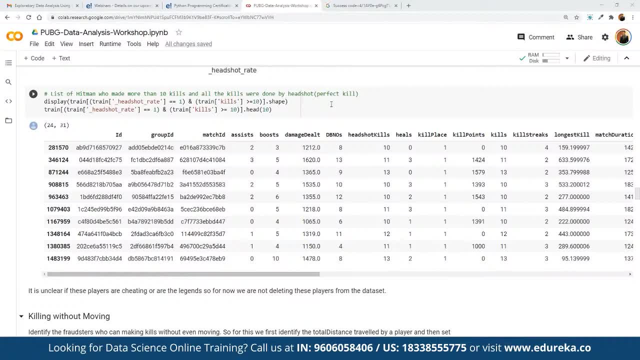 in the pin as a part of the headshot kill. So we had to find out that by using the same train data set and then here we can find out the headshot rate, where headshot is going to be one. Now, This is going to is something that we are going to derive out of it. 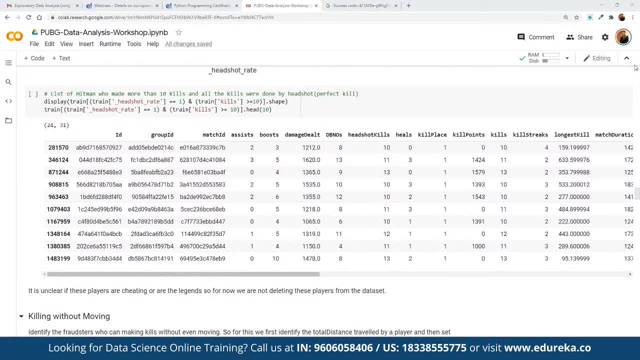 So here we can define: Okay, what is the headshot rate for a for every data pointer that we have in the current data set, and if the headshot rate is one, that means if every kill the player has has been done using a headshot. 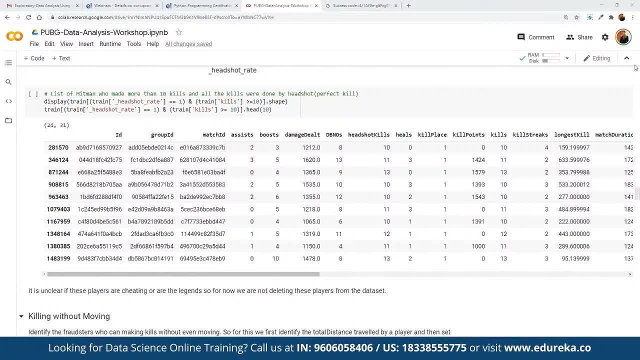 then we are going to drop these values as well. So every every kill done by the headshot, and plus where the kills are more than 10.. So here we can see how we have 24 rows having this kind of data pointers. same way. 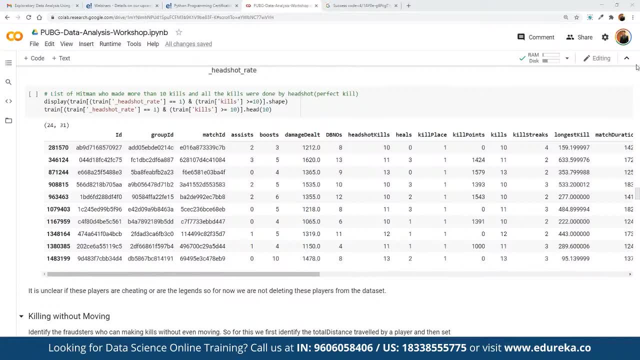 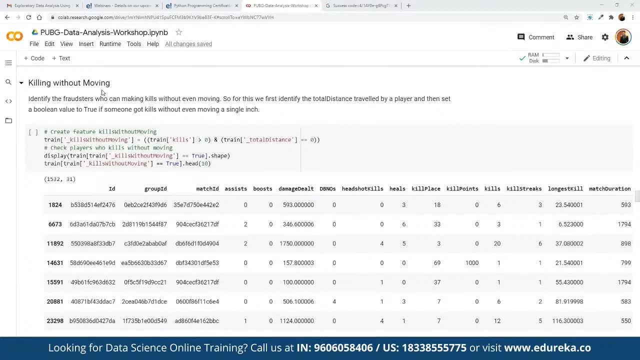 We may have different type of outliers. Let's say, here we have to find out those players who have made a kill without moving a single inch. Now we know that this is also not practically possible, So now again, we are going to find out those players. 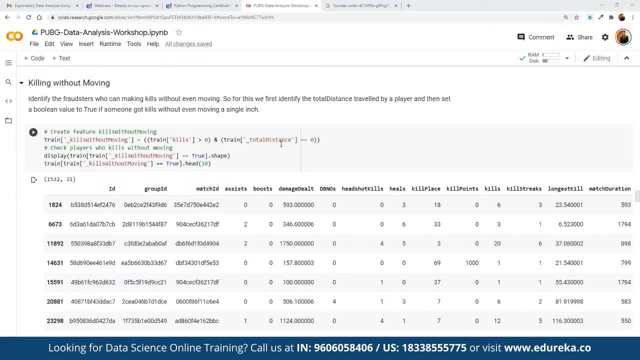 who are having kills more than zero, where the total distance traveled is also set to zero. So when we so, once we run the statement, we are going to see there 1532 rows having this kind of data set. So we know that practically it is not possible.